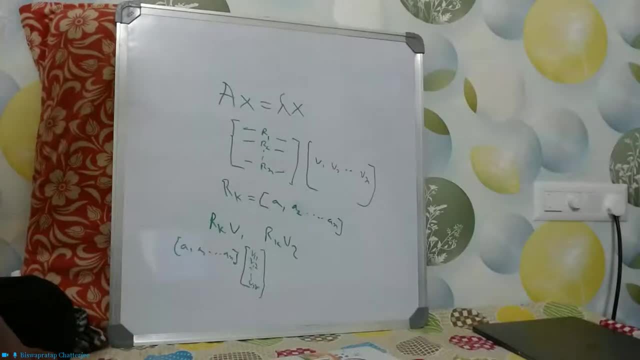 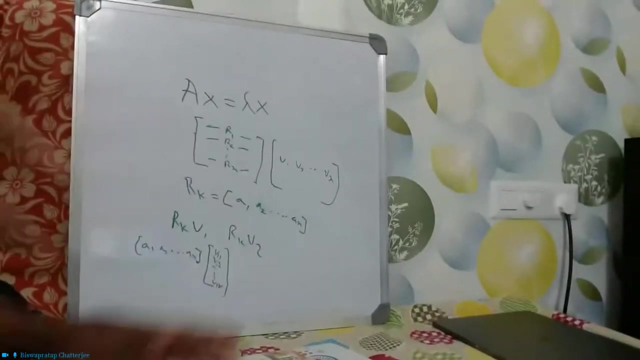 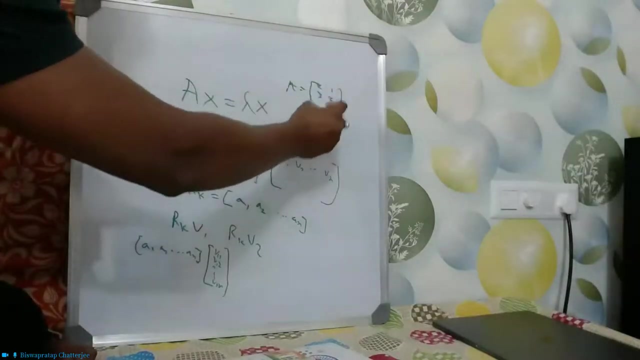 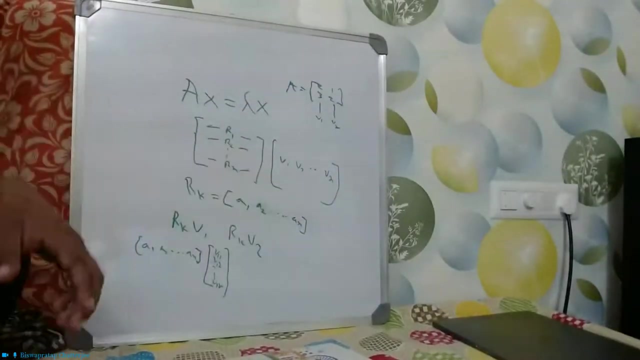 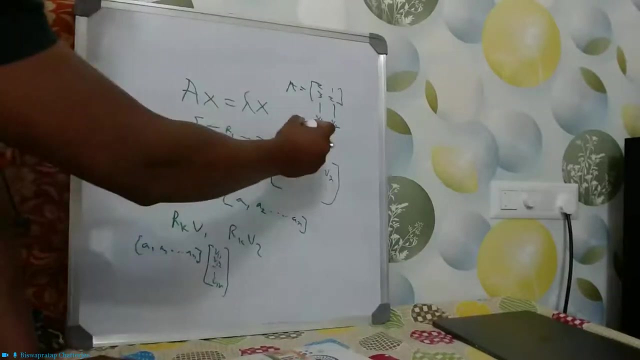 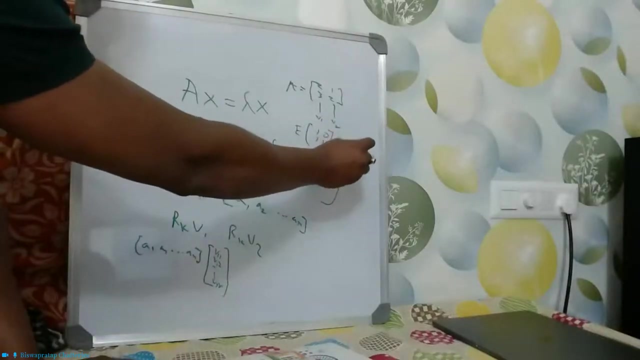 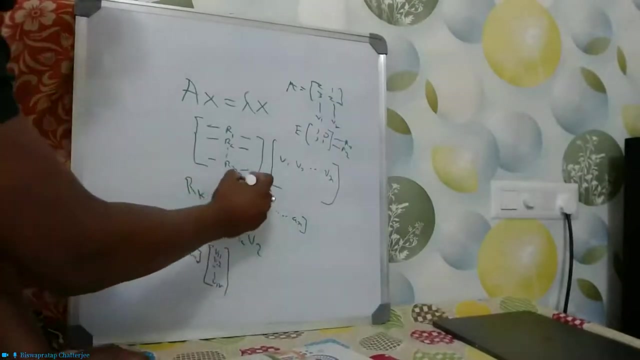 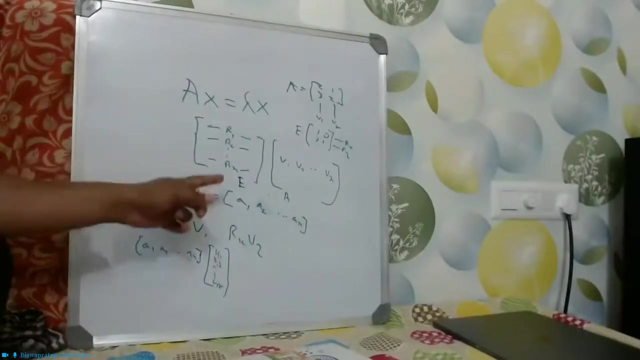 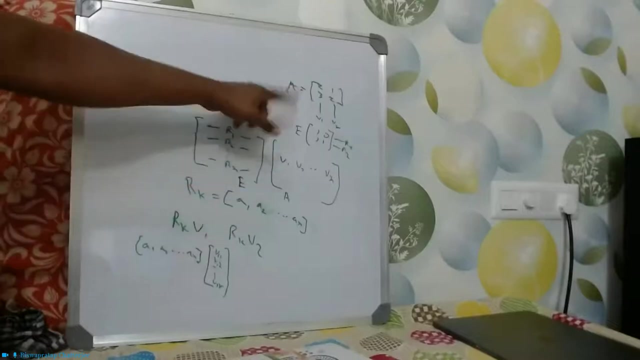 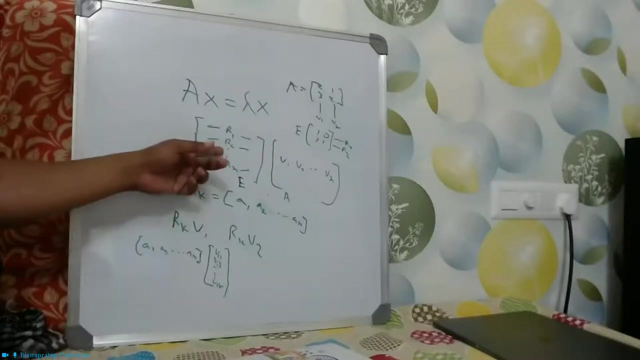 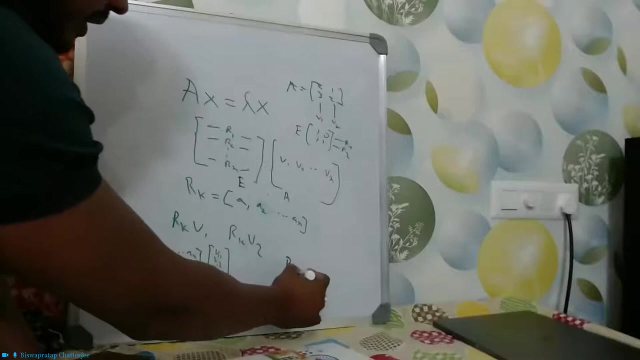 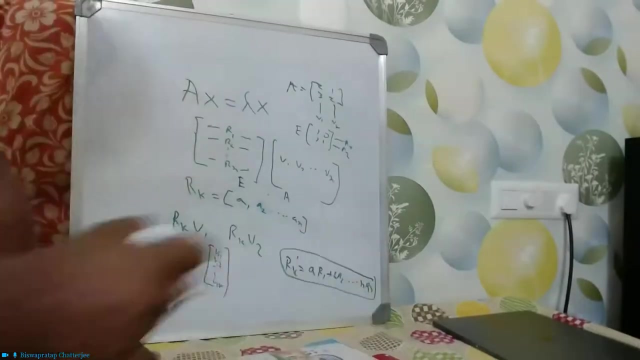 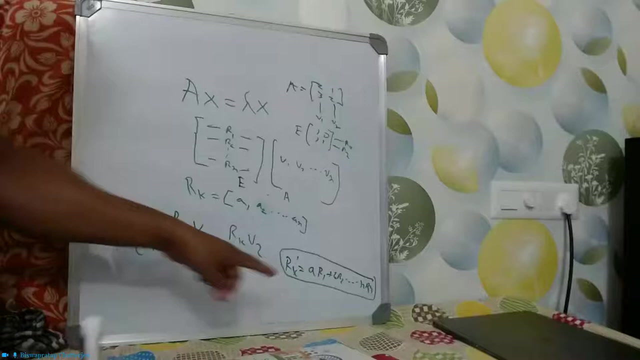 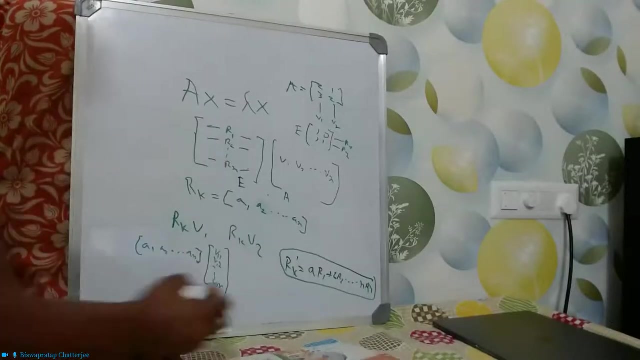 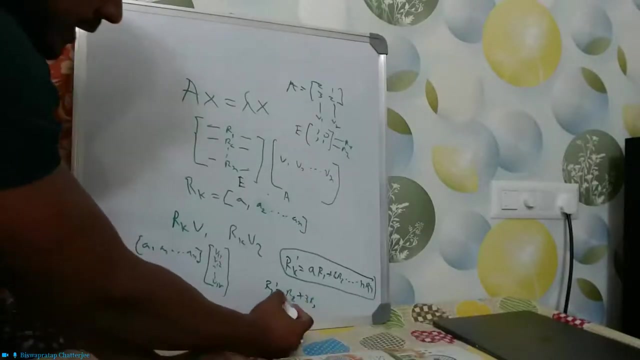 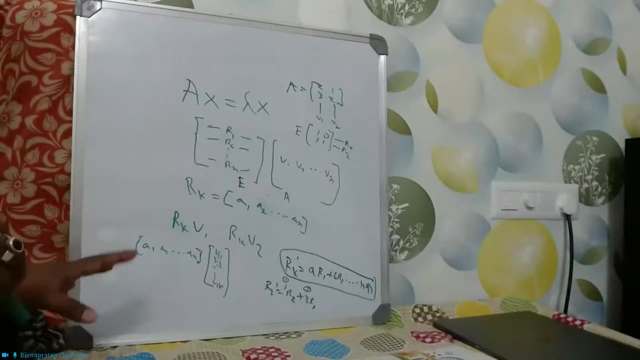 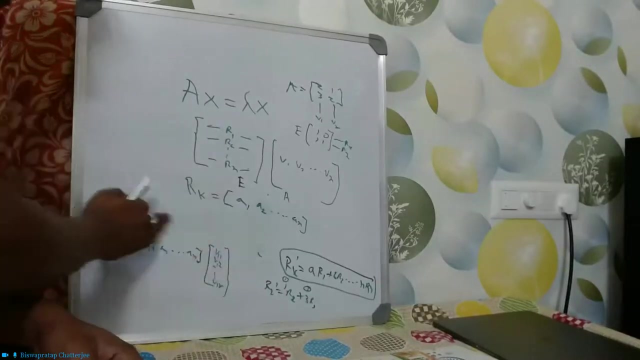 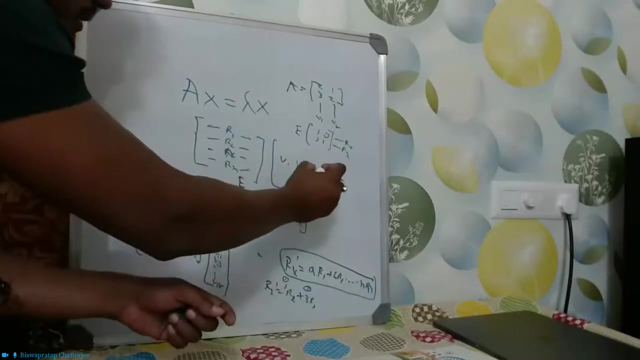 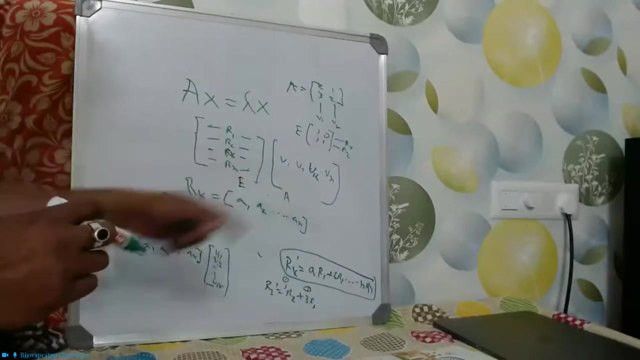 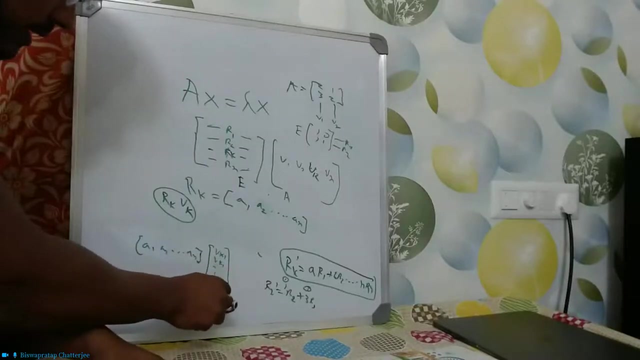 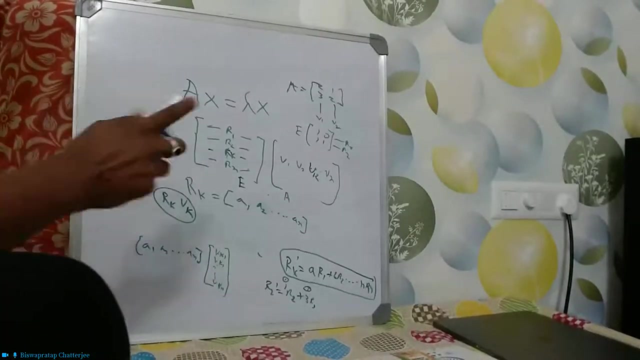 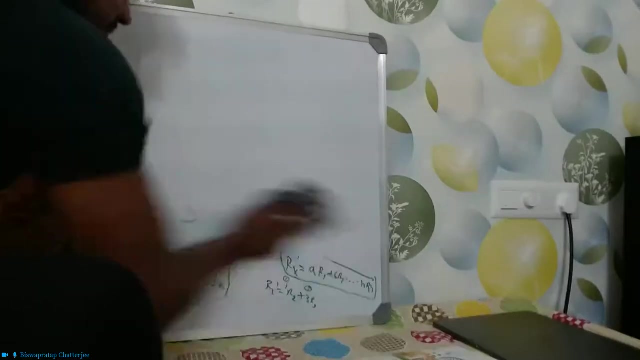 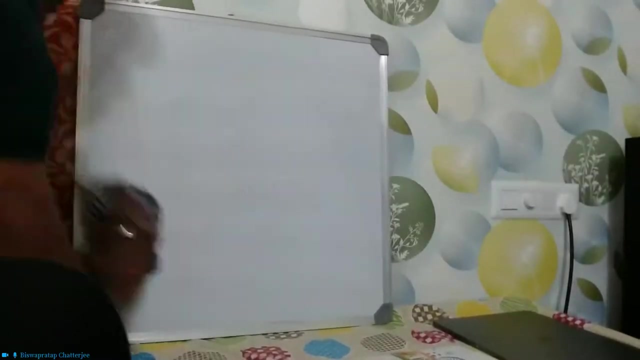 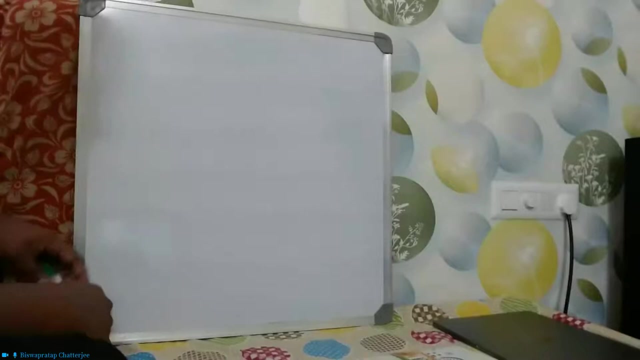 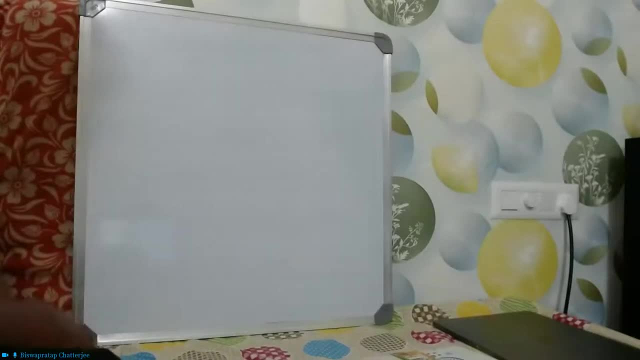 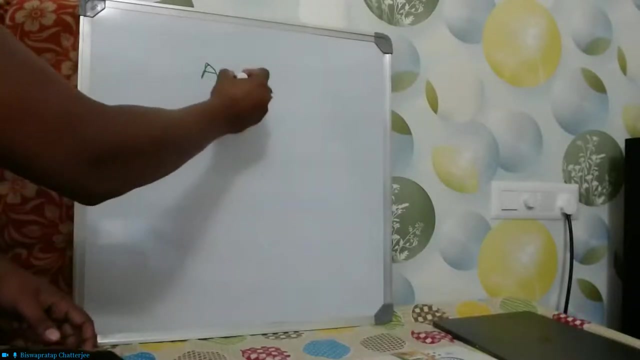 But if it is rotating, then any vector multiplied with that new rotated matrix it will have different eigenvalues and eigenvectors, right? So that is the philosophy that I am taking in mind and starting my proof. I want to see that, whether A, the matrix A, with which our necessity is what? 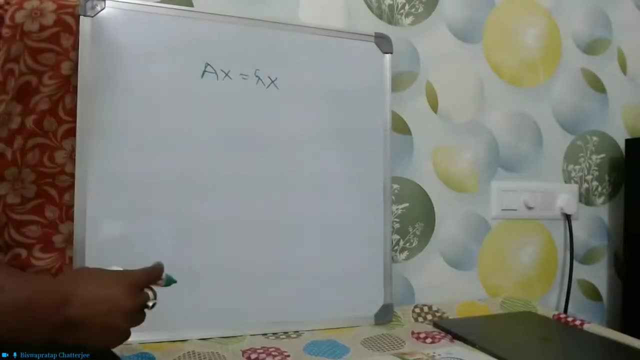 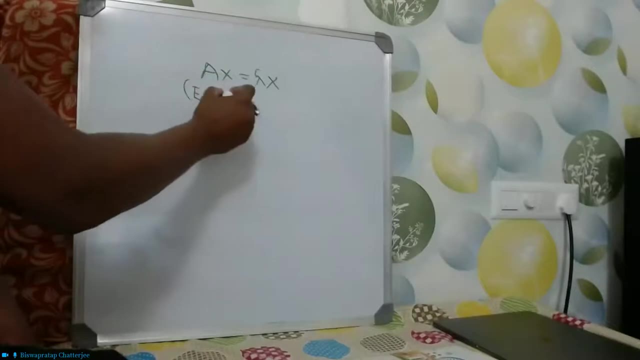 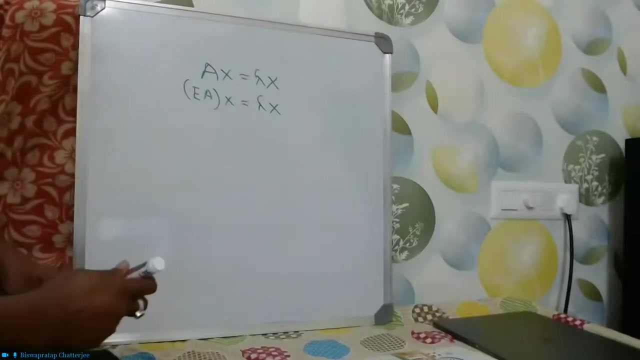 Ax is equal to lambda into x. If this happens, then we know that it is true And we want to. we want to prove that EA x is equal to lambda into x. If this is, if this happens, then we will say that. 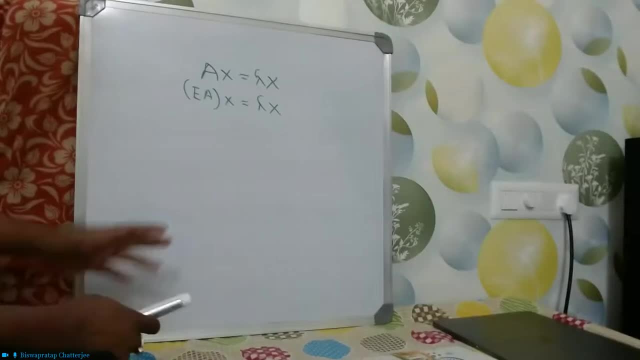 okay, the eigenvalues do not change. and eigenvectors? we will see it changes or not, but at least eigenvalues do not change. Okay, so this is our concept. This is what we want to prove or disprove. Okay. 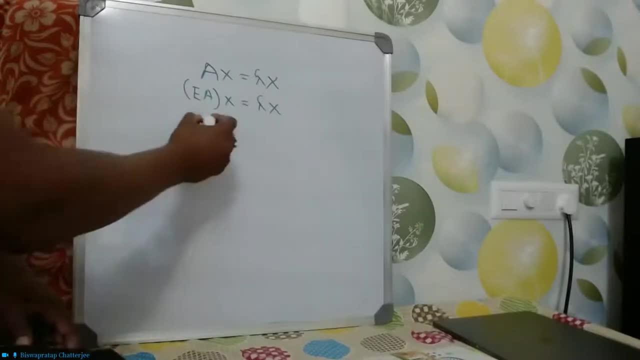 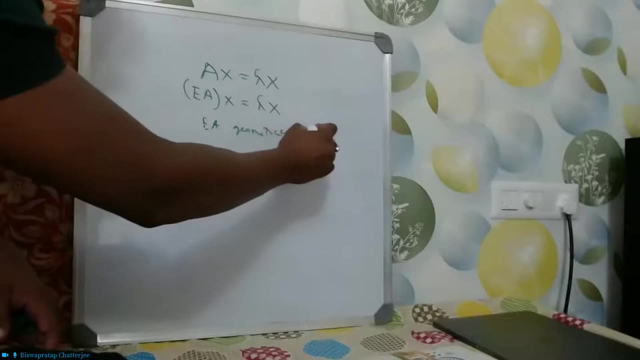 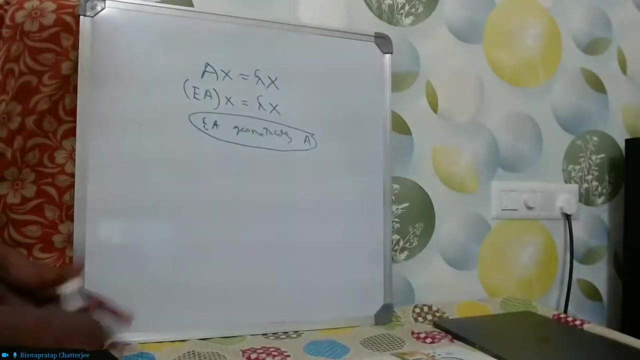 So now this EA matrix is important, Whether this EA is geometrically equal to A or not, okay. Geometrically equal means the same matrix can be scaled up, scaled down, okay, But geometrically they are same, okay. 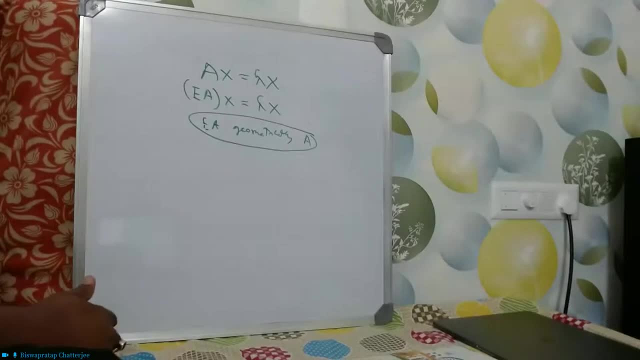 A matrix can be a combination of vectors And out of these vectors, one vector is scaled up or scaled down, So I can say that it is okay, geometrically same. So when I, when I find, try to find the eigenvectors of that matrix, 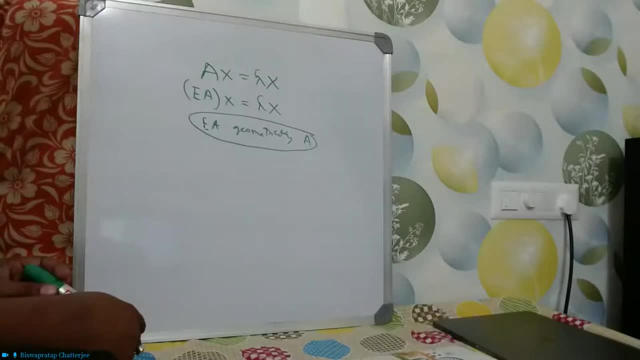 then I can have the same eigenvectors. Maybe that way those vectors will be scaled up, scaled down. The values of the vectors will be eigenvalues will be scaled up, scaled down, But they can have the same eigenvalues and eigenvectors. 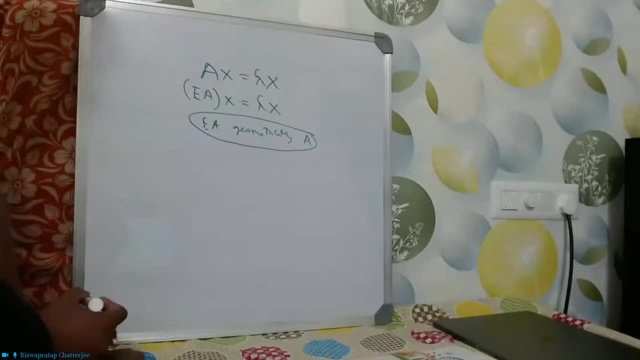 Okay, To prove that. to prove that what I take a general case of EA x. So EA x, EA x R1, R2, dot dot dot Rk, dot dot dot Rn. okay. 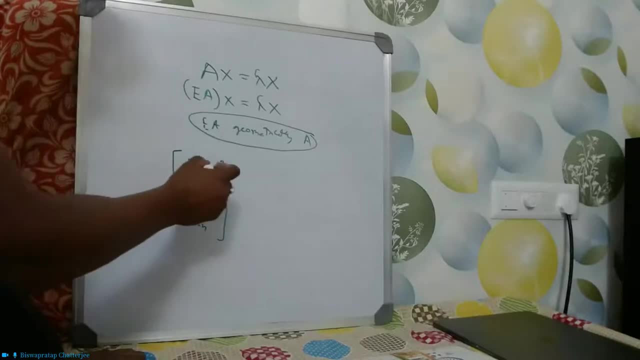 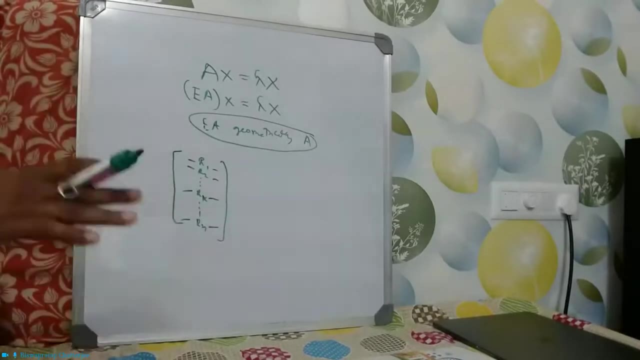 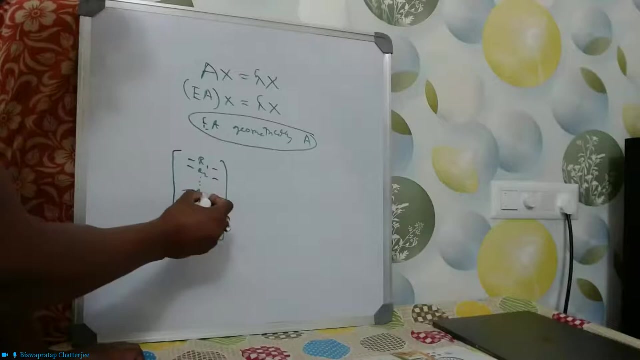 I take the E matrix in this form. okay, So R1 to Rn. okay in general, And there will be a in generic. we can say Rk or I will write Ri. okay, So Ri is any one row of the elimination matrix. 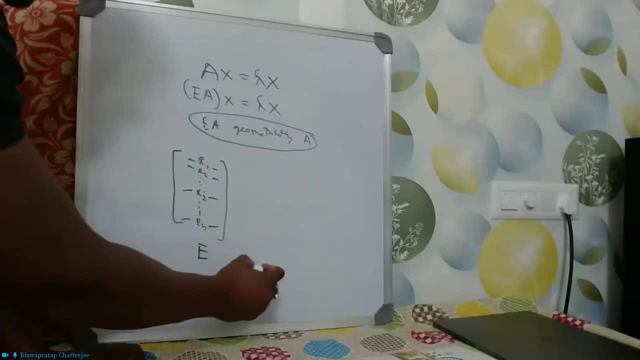 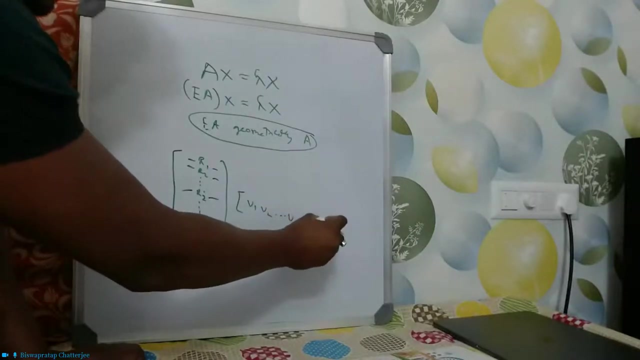 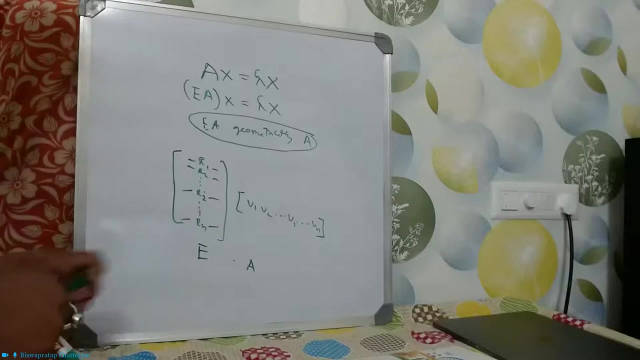 So this is E And I am multiplying with A. So in that way, I also took A as a horizontal matrix where V1,, V2,, Vi and Vn- okay, So this can be a situation where I, when I am multiplying E with A, okay. 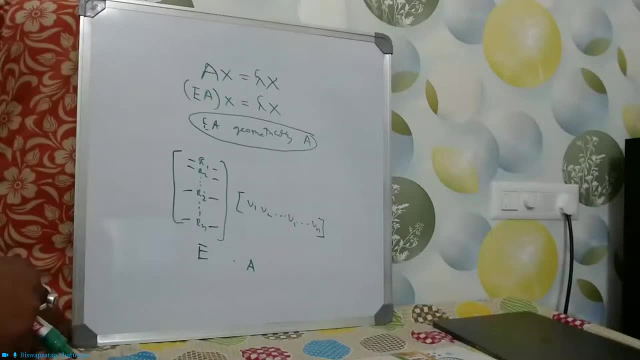 This can be a situation, And when I am multiplying this one, what? although R1 is a function, it is a full blown row and V1 is a full blown column, but still according to our rules of multiplication, hm, if we take the outer product multiplication rule. 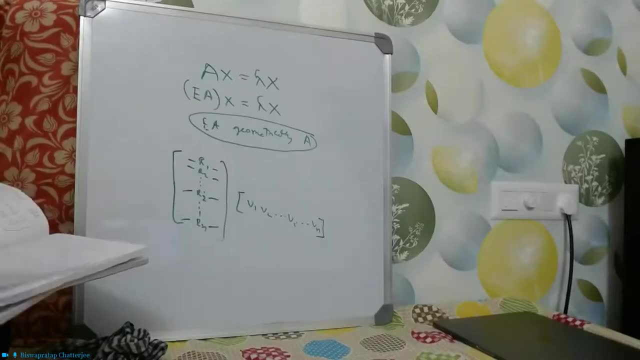 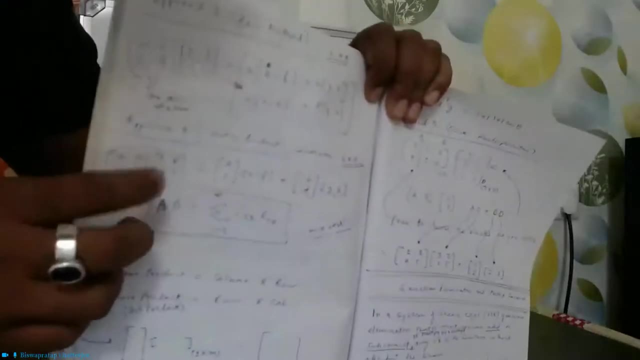 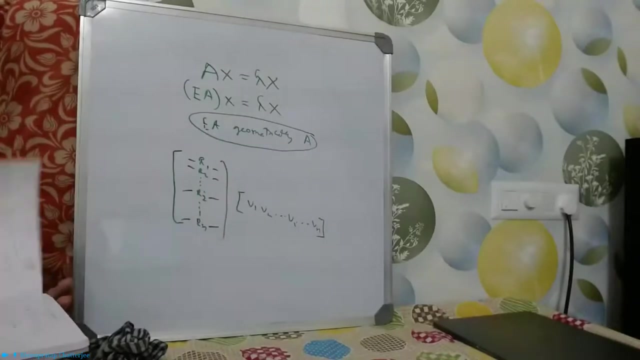 if you remember that where outer product multiplication rule, this one, this one, okay. If we take the outer product multiplication rule, then ah, or the inner product, any one you can take, okay, And so, or this one, the dot product, okay. 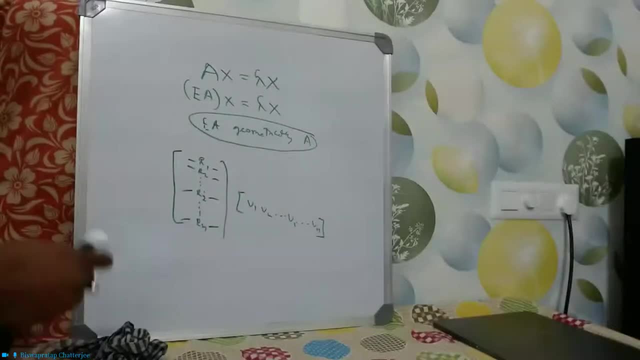 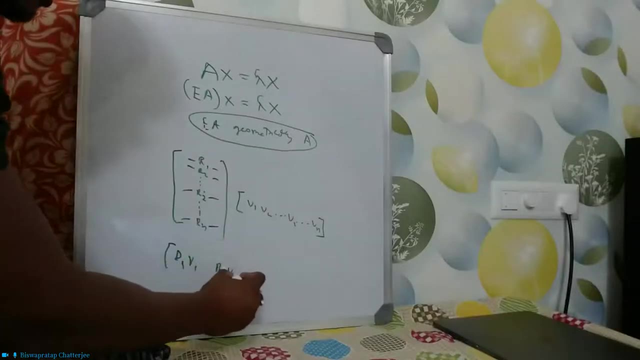 So what happens? This multiplication result will be this: one's result will be R1, V1,, R2, V2,, similarly, Rk, Vk and Rn- Vn. So this will be the multiplication of these two matrices. okay, 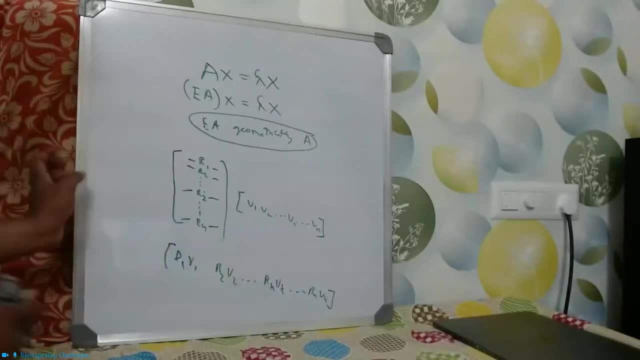 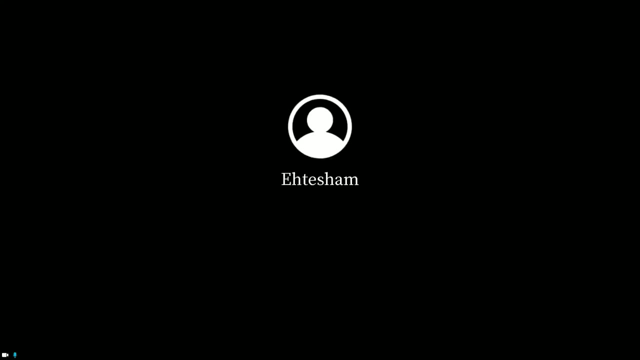 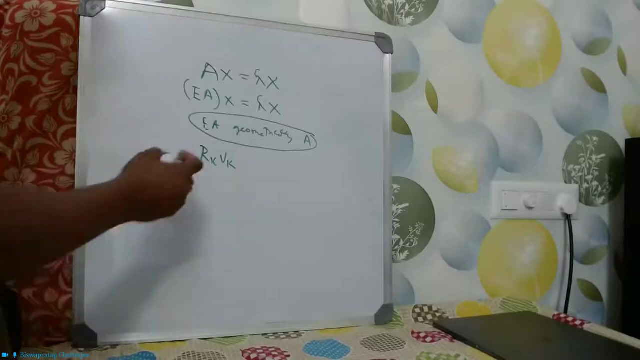 Now we are interested in a generic Rk Vk. okay, So we go to a generic Rk Vk. You are solving the first question, right, Biswa? Yes, yes, yes, So we go to a generic Rk Vk. 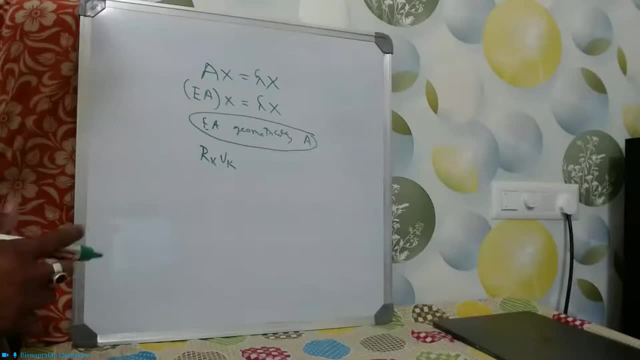 and then we see what. what happens here. So I can take Rk Now Rk, what is Rk? Rk was one of the rows of the elimination matrix. one of the rows of the elimination matrix. How does we write an elimination matrix? 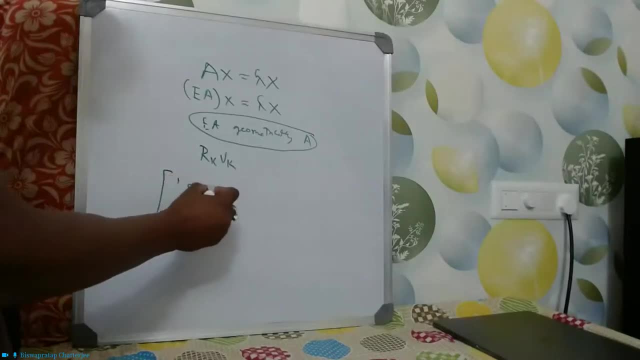 Suppose we do not want to change the row 1, then we write 1, 0, 0, like this. Suppose we want to change row 2, as row 2 is equal to row 2, dash is equal to row 2. 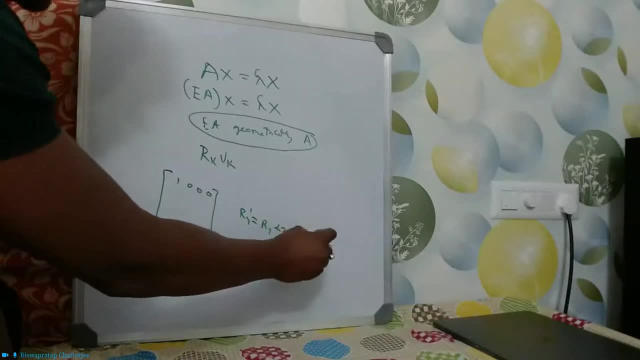 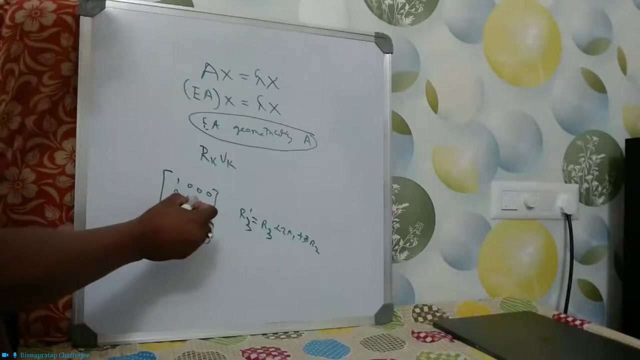 plus 2, row 1 plus 3, ah, ah, row 3 is equal to row 3 plus 2. row 1 plus 3, row 2: like this. We write like this, right? So what happens? We do not change the row 2, so 1, 0, 0, 0, but we change the row 3.. 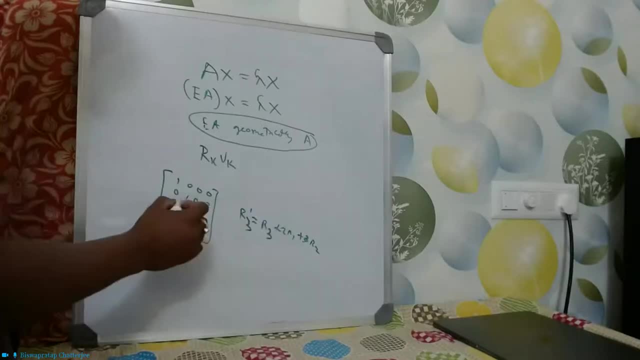 So in that case, row 3 will be 1 plus 2, row 1, 2, row 1 and 3, row 2, 3, row 2 and 0.. So, like this, others continue, So we are considering this one okay. 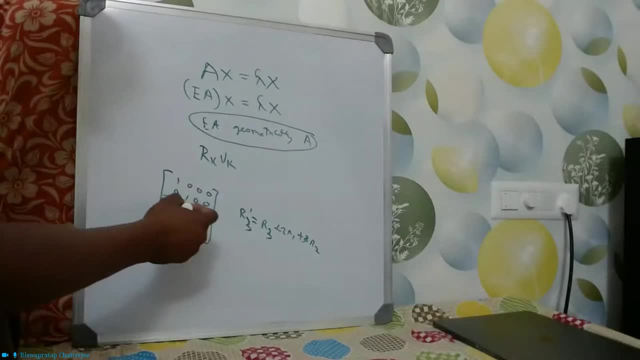 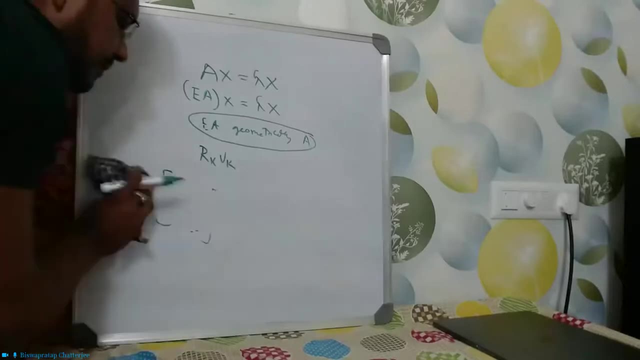 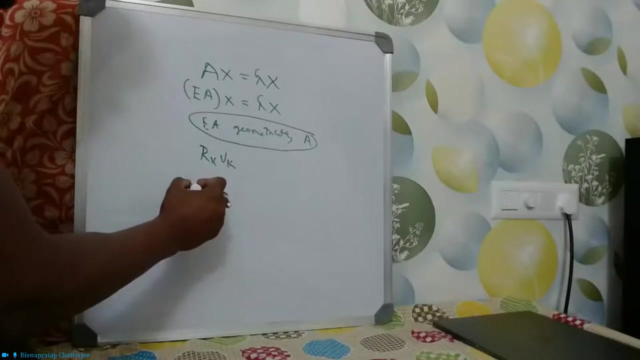 What is this? This is a linear combination of real numbers, right, So I can choose our Rk? Rk I can choose as sorry r not k? r i r? i. So I can choose my r? i as r? i a r i b like this r i n. 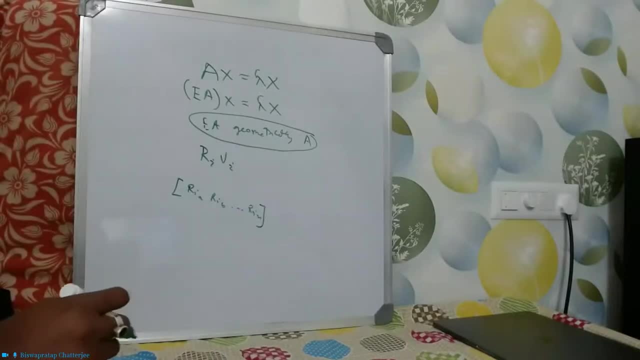 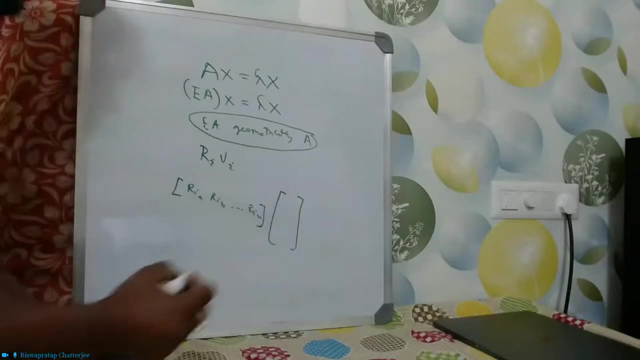 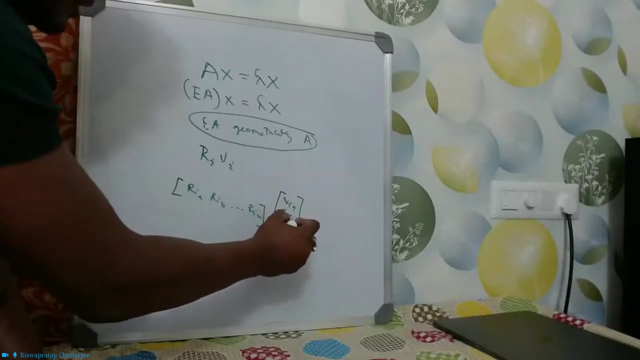 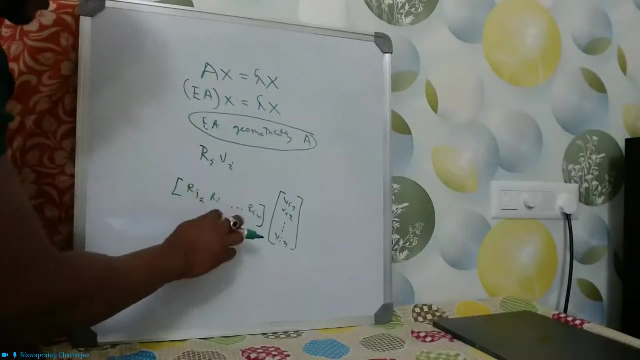 I can choose like this: right, I can choose like this: my r? i and v? i. similarly, it will contain ah. I can break it horizontally and like this, I can write So v? i will be like v i 1, v i 2 till v i n. this is r i 1, r i 1, r i 2 till r i n. okay. 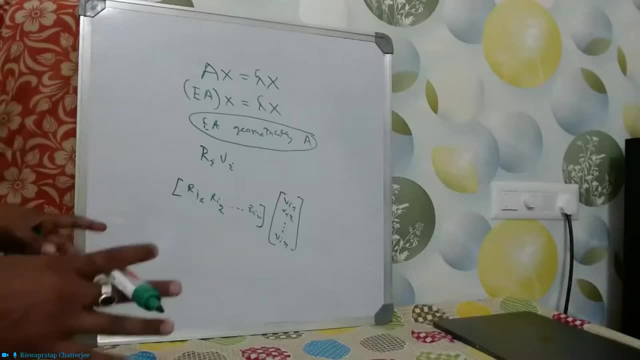 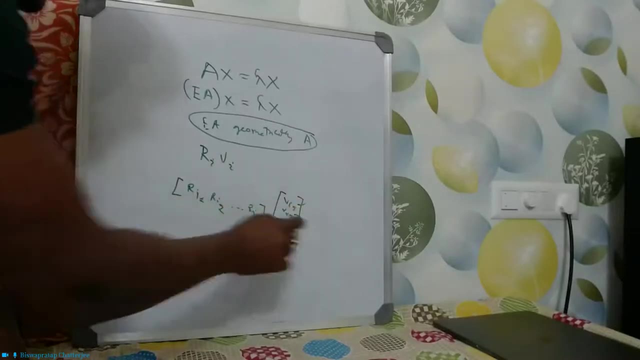 So this is my broken down piece of r i v i. okay, Now what I see is that every vector r? i 1. r? i 2. r? i, 3. r i, 4. r? i 5.. 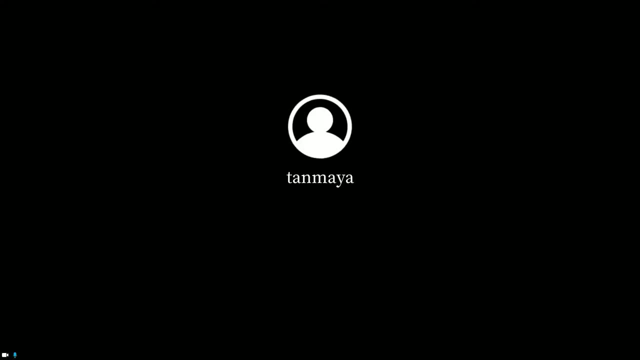 r i 6. r i 7. r i 8. r i 9. r i 10. r i 11. r i 12. r i 13.. So this r i one is. it is nothing. row number r, column first right. 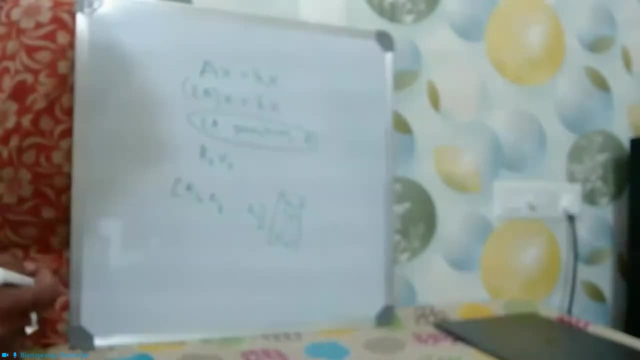 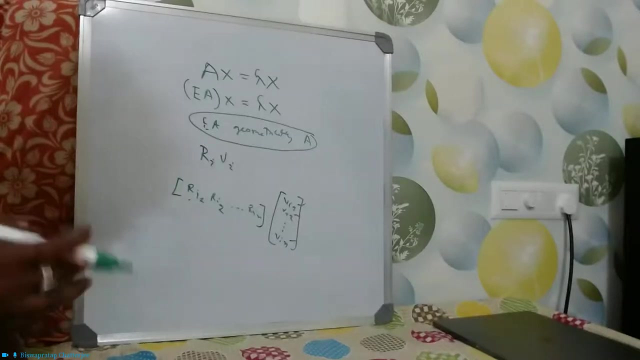 Yes, yes, yes, it is a coefficient, because we saw that right. a row, an elimination matrix, is a group of rows and each row can be a linear combination of the other rows. That is what is an elimination matrix definition, right. 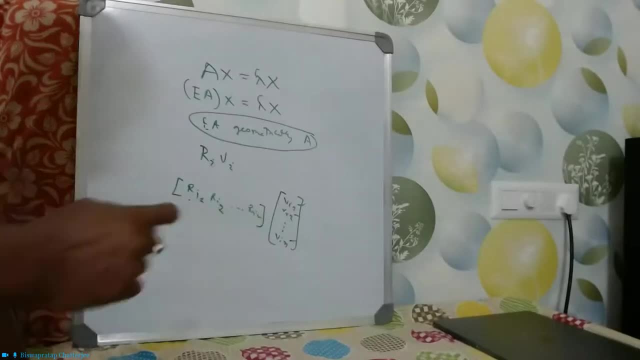 So this r i 1, ri 2, ri n is the coefficients of linear combination of any row. ok, So suppose I have this. this is a sample elimination matrix. I keep the row 1 same. I change the row 2. 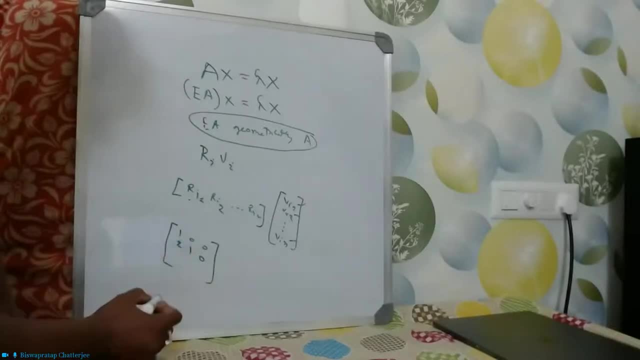 like this. and I change the row 3 like this: This is a. this is this can be a. this can be an elimination matrix in our Gaussian elimination right. I am keeping row 1 same. I am multiplying. I am multiplying row 2 with 1 and adding 2 times of row 1.. I am keeping row 3 as row. 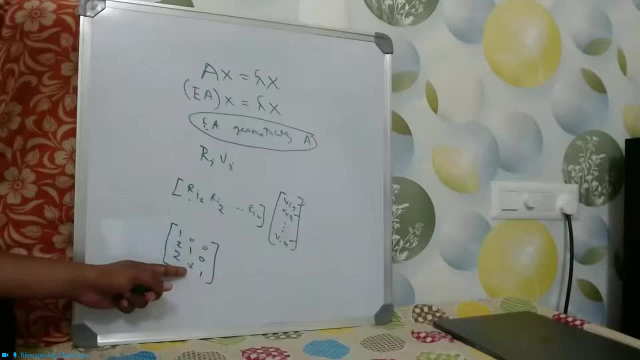 3 plus minus 1 times of row 2 and plus 2 times of row 1,. ok, So this can be a generic elimination matrix. So if I take in general elimination matrix, I am keeping row 1 same. I am keeping row. 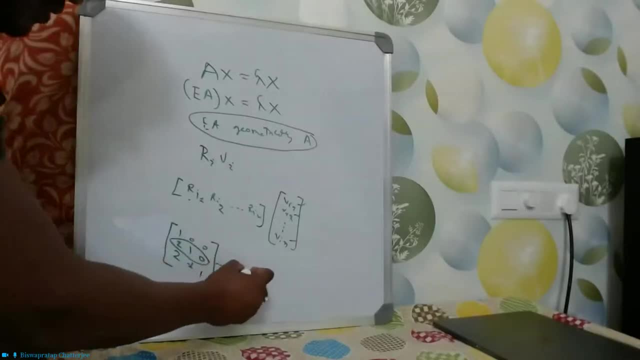 2 same. If I take out any one of these, then this is what 2, 1, 0 like this: What is 2, 1, 0?? These are the coefficients. these are the linear combination coefficients of each. 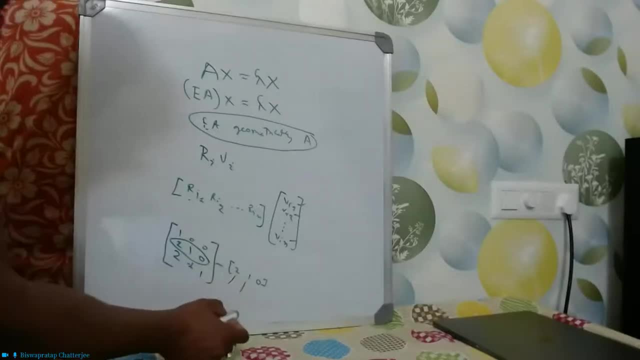 so 2 times of r1,, 1 times of r2,, 0 times of r3.. So if I can write this one as a, b, c, this is also fine. So this is same as this one. this a. This can be a. this can be b. 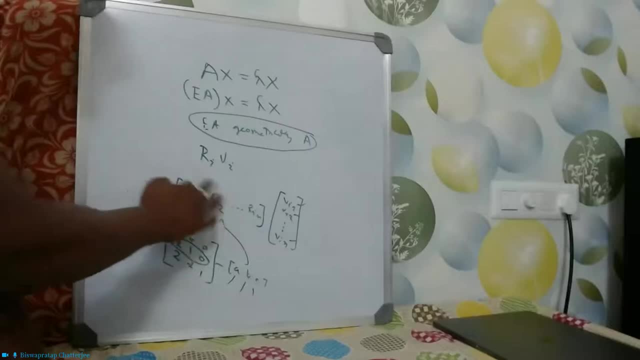 this can be: c: R i th row R. this is R i th row in the R i th row. this is: R i 1 is the first coefficient. R i 2 is second coefficient. R i n is the third coefficient. ok, So now what I see is that I am multiplying a matrix with another matrix, where these are: 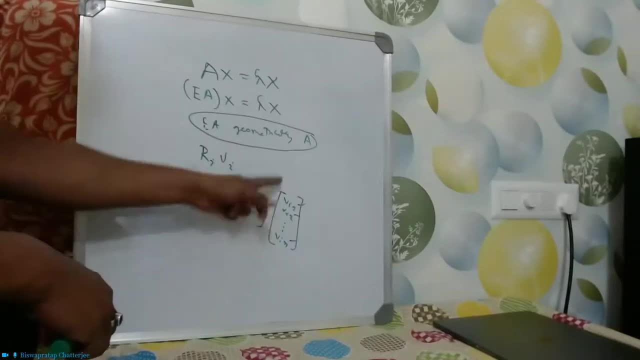 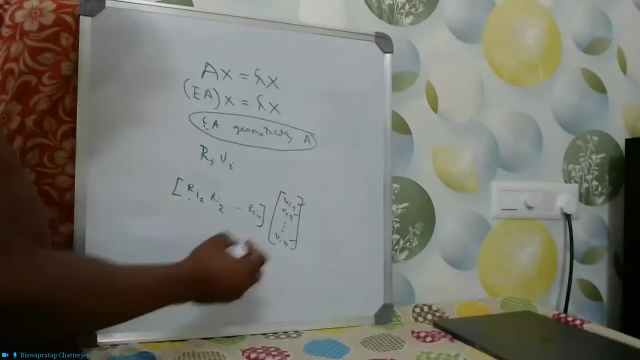 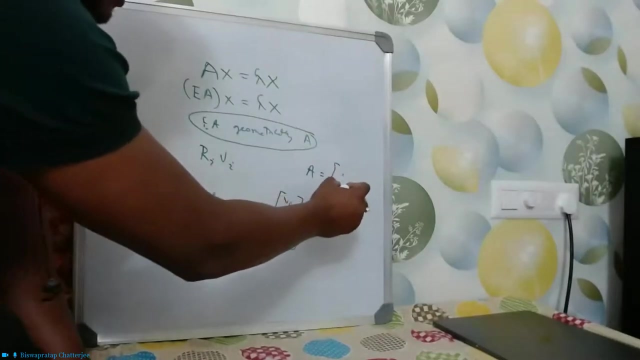 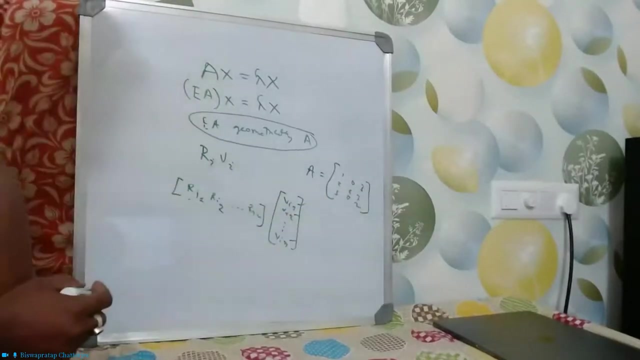 the vectors vector. what is this? the vector components, right? So suppose my? this is very important understand this. So suppose my a matrix. a matrix is 3 dimensional, ok, So 1, 2, 3, 0, 1, 0, 2, 2, 3, 3, 2. ok, Suppose this is my a matrix. what do I understand from there? 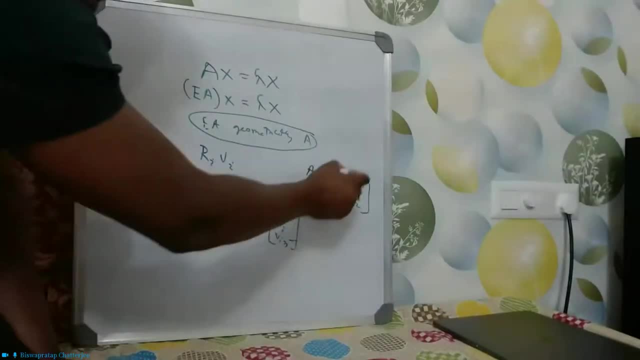 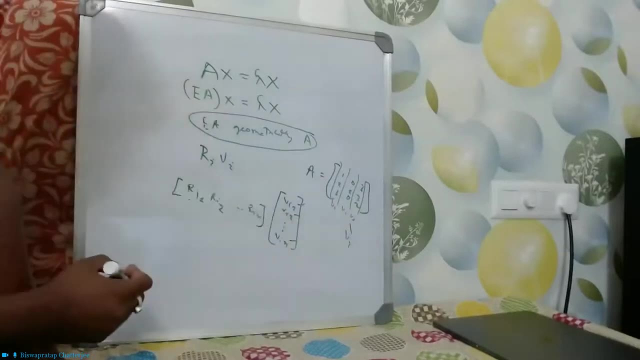 this is combination of 3 vectors. Ok, v 1, v 2, v 3. now let us take this v 3 as v i in our case. ok, Now this v i has 3 components: 3, 3 and 2. what does that mean? the v i in the 3 dimensional plane is represented by 1- 2. 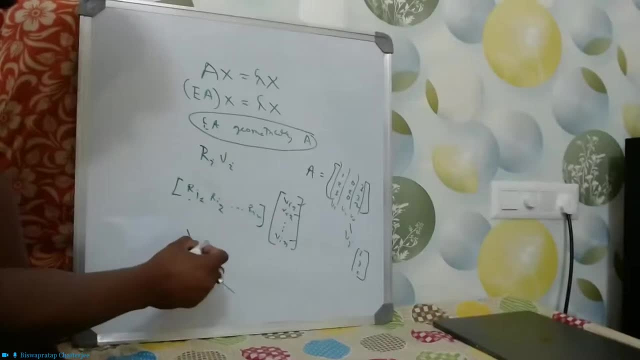 3 1 2, 3, 1, 2.. So this is like some point here. Now, if I have take v I and v 1, this formed out from v i, this one, ok. So this is I. take v i and v 2, this one, ok. So this is the components of v i. So v i, I 1, i 2 till I n is what this? 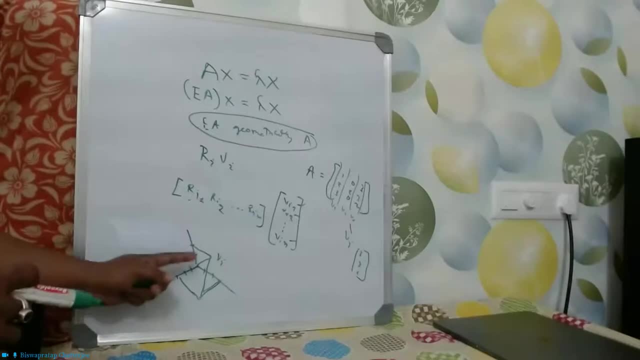 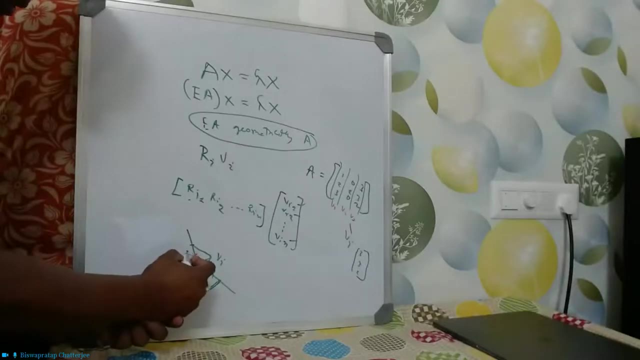 one. So this is our v? i right and vi 1, i 2 till I? n is what this one? I 1 is 3, i 2 is 3 and i? n is 2. ok, So these are the components of v? i which are for a linear combination. 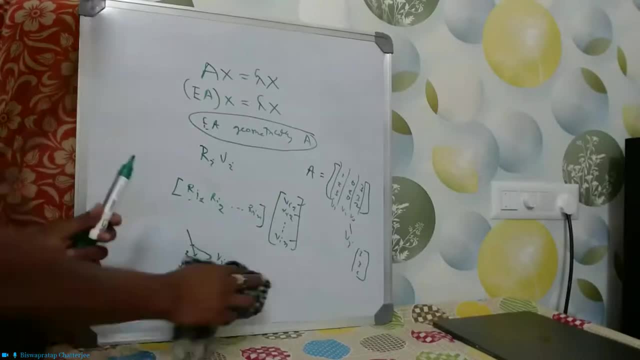 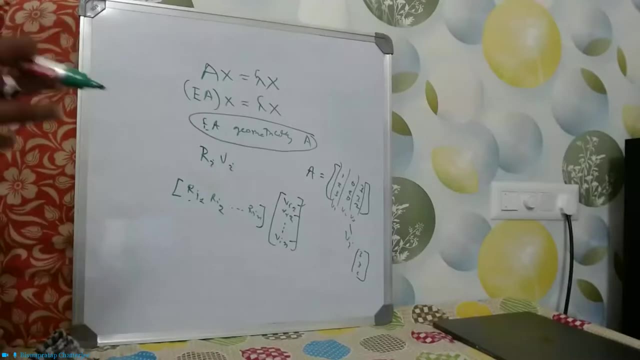 of the i cap, j cap and k cap vector. ok, So what we know, any vectors can be represent as a linear combination of the v i. So v i i 1, Keeping, we know, between this i cap and combination of the i cap, j cap, k cap, d l cap, m cap, right any dimension. So I have written. 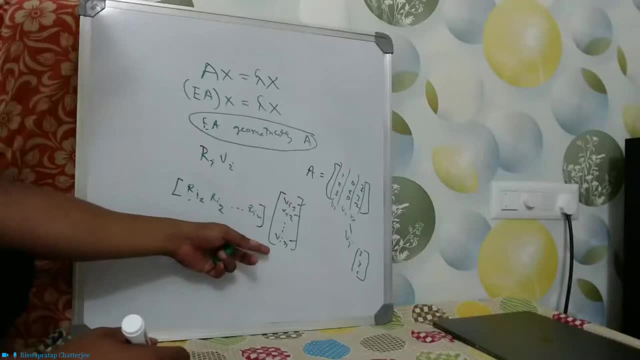 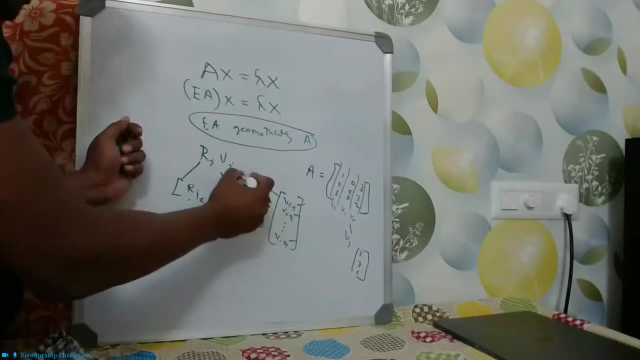 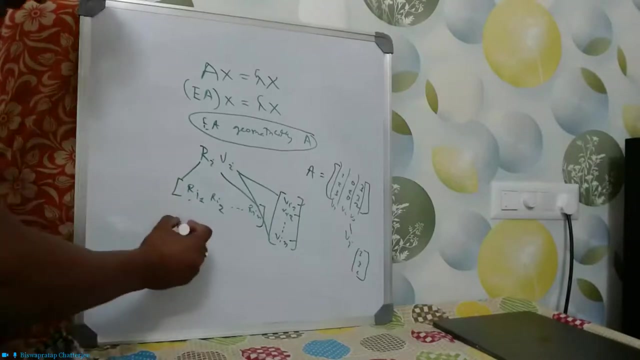 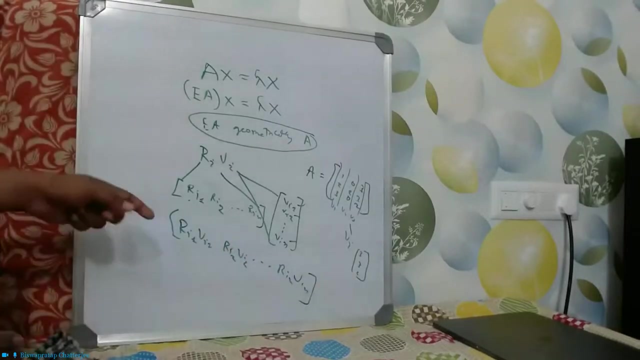 the components of each of the vectors in the in this format. So I have opened up ri and I have opened up vi ok into its individual components. So when this multiplication happens, what happens? ri1 into vi1, ri2 into vi2 and, like this, rin into vin. So what I see is that I am multiplying. 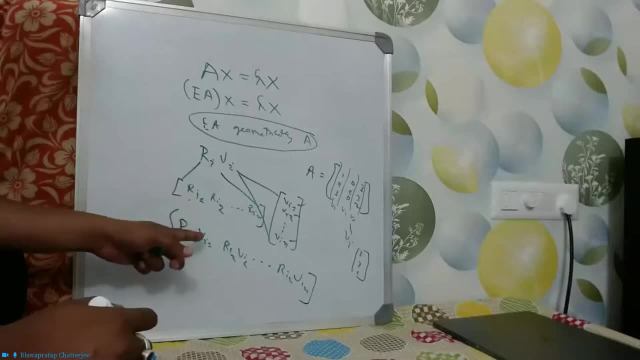 a scalar value. So ri1 is a scalar value and vi1 is also a scalar value. So I am multiplying two scalar values where vi1 represents the component of vector v in the x direction, component of vector v2, v in the y direction and similarly in the nth dimension. So I am multiplying a scalar. 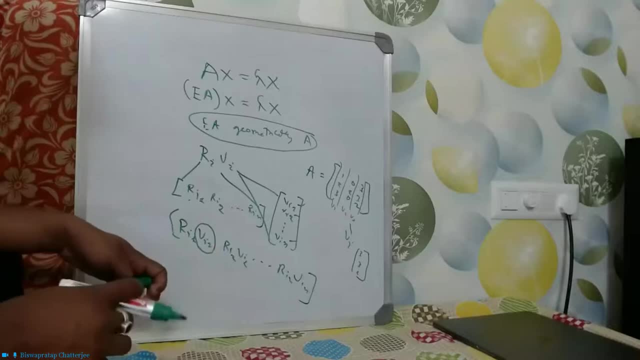 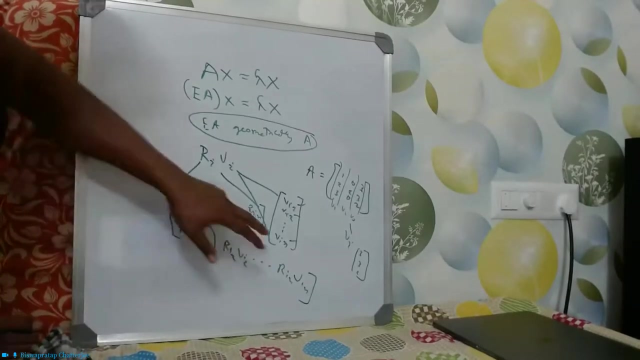 to each of the component of v in all its dimensions. ok, Now if all these scalars ok are same, like 2, 2,, 2, 2,, everything is 2, same, Then what happens? Then this vector is scaled up. 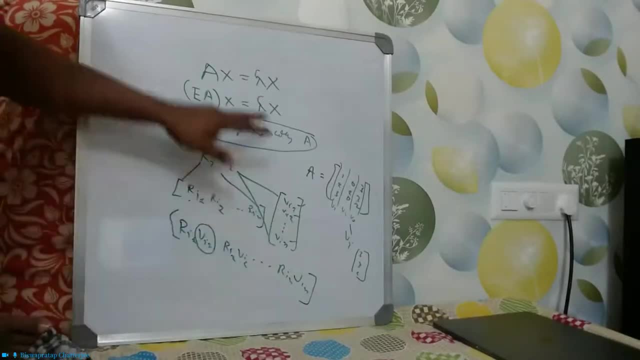 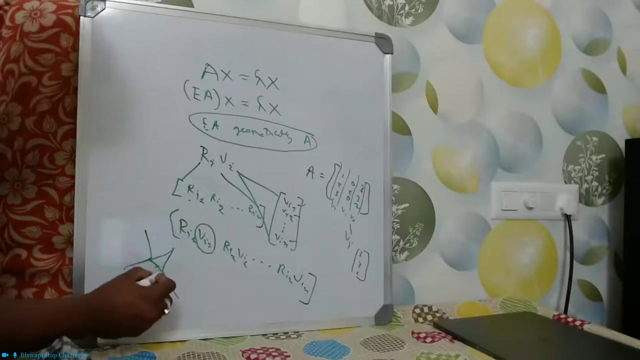 uniformly. So in our matrix A this vector is scaled up uniformly. ok, All its components are increased by 2 times. So earlier if it was like this, 3, 3 and 2, and now it will be scaled up: If r- i is 2, r i- 2 is 2, everything is 2,, 2, 2 and it will be 6 times, 6 times. 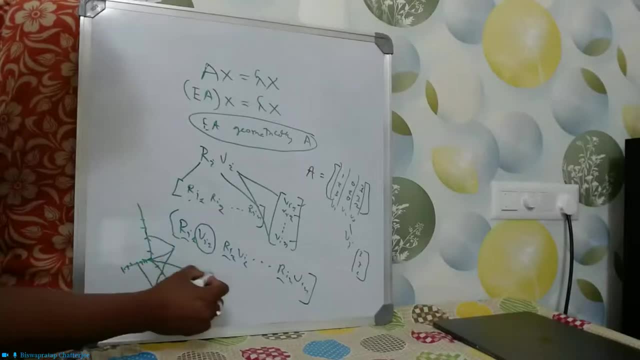 and 2 times. So this vector will be something like this: scaled up 2 times, ok. ok, So this is the first vector and after that, scaled up 2 times, this is the second vector. ok, So that can. 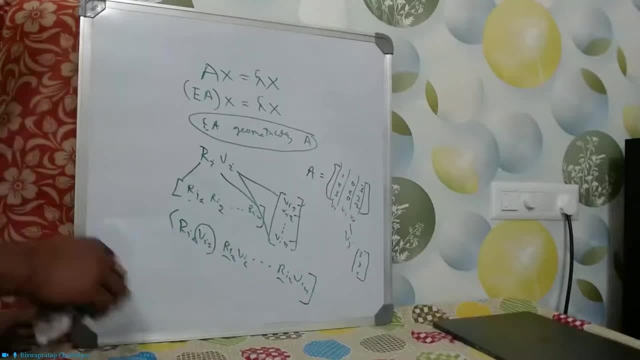 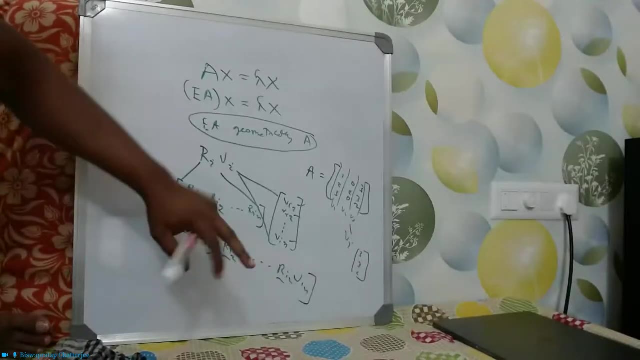 be one case or another case can be that r i and r i 2 and r i n are different values, So each component is scaled in a different way. Some the x component is expanded 2 times y component, So x component is 3 times n component is expanded, say 20 times. ok, So in that case 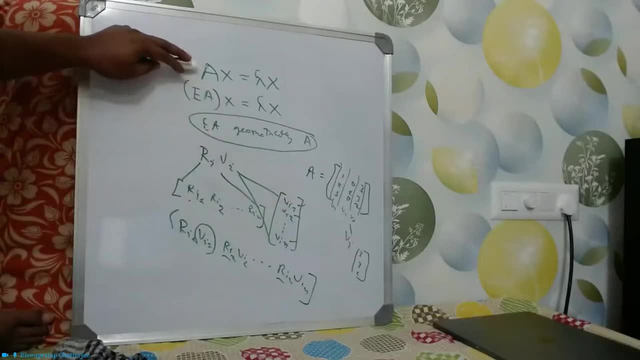 what happens? Our v vector, which is a component in A- ok, is completely changed. Our v vector is completely changed, and in case of equal, also our v vector is changed, ok, So in both the cases our v vector is changed. 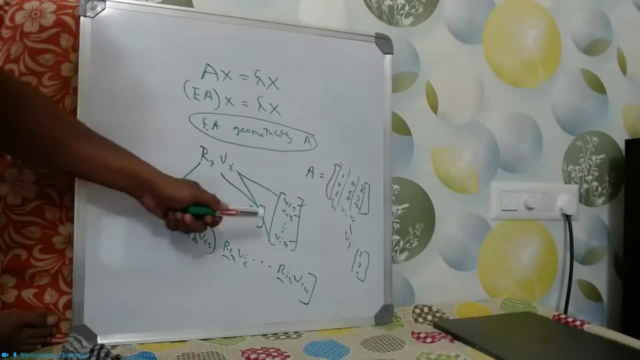 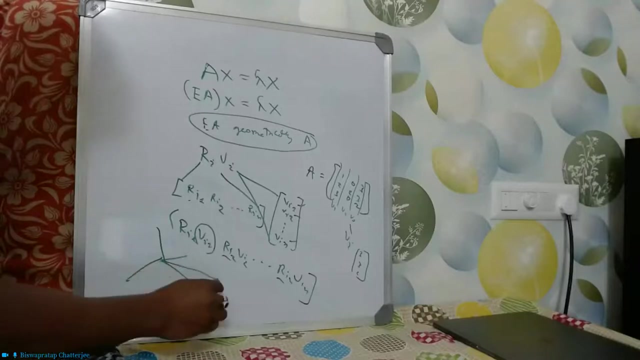 row eliminations matrices. the components are same. also it's changed. if it is different, also, the v vector gets changed. i showed you right. when i scale a vector two times, it changes the angle. right, it is not in the same angle anymore. okay, if it is like this. after scaling it becomes like this: 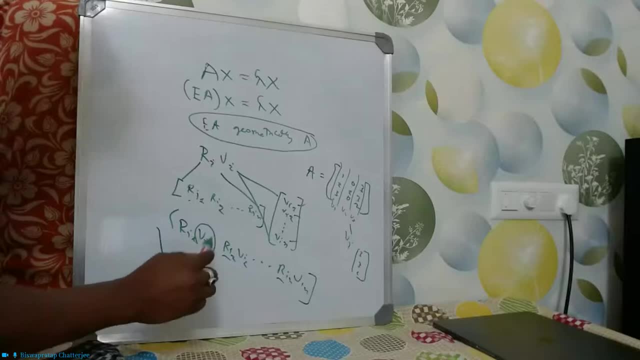 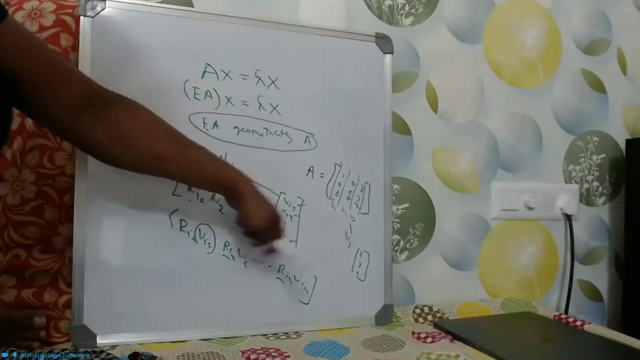 okay, so there is an angle that happens between them, right, so they don't direct in the same direction. and if it is scaled differently, then then definitely the angle is changed. so since our a changes, okay, our a changes, and out of a one of the vk we showed that it changes. 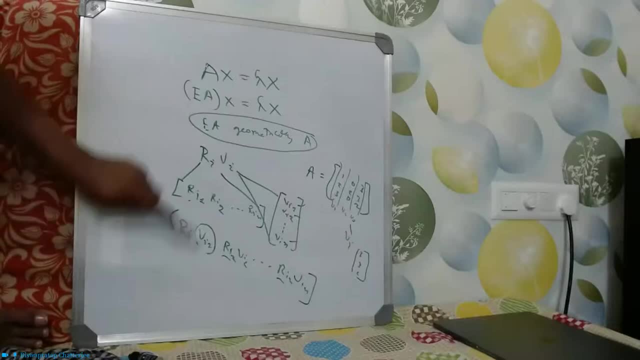 now, multiple vk also can change because of the nature of e. so in that case our a matrix, after multiplied, getting multiplied with e- does not change, remain the same matrix anymore. okay, it changes into a new, different matrix. and this new, different matrix will not have the same eigenvalues and eigenvectors as the old matrix. okay, so ea is not. 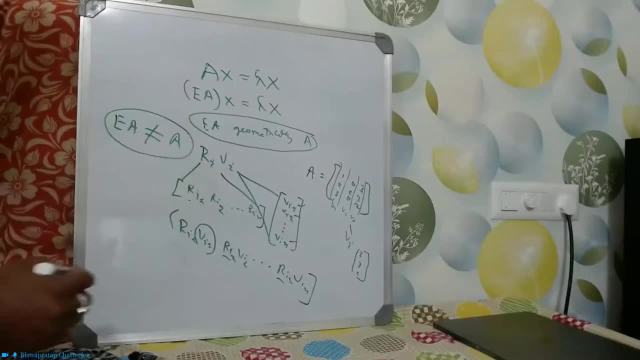 geometrically equal to a. okay, because we saw that after multiplying with e, our a matrix completely changes. it becomes a new matrix which is not geometrically equivalent to a. okay, so in that case, what will happen? all the eigenvectors of a and a will not be same as the eigenvectors of ea. it will be different. so when you multiply, 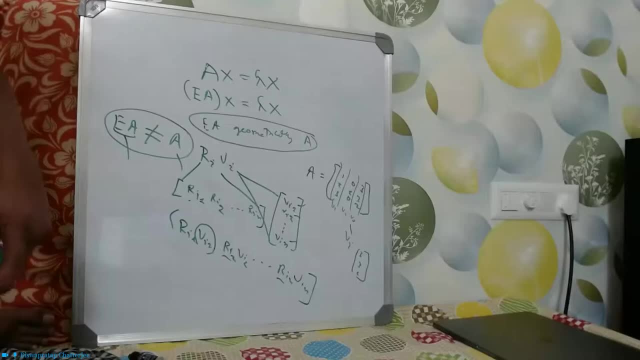 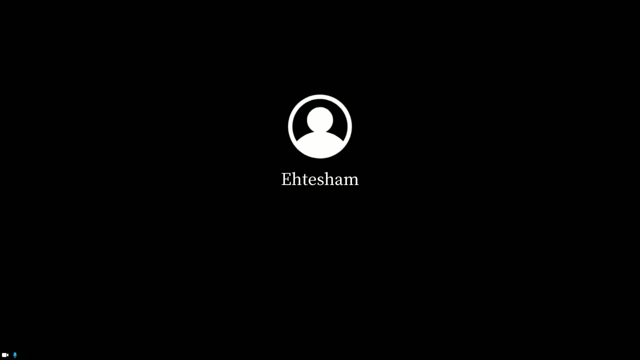 an enumeration matrix. with a matrix, then the eigenvectors and eigenvalues change for that matrix. any doubt is no, this is fine. also, you got it right. huh, yeah, I got it. there is one more point, like since we know that, like we don't have inverse right, like a minus, i lambda emeee. 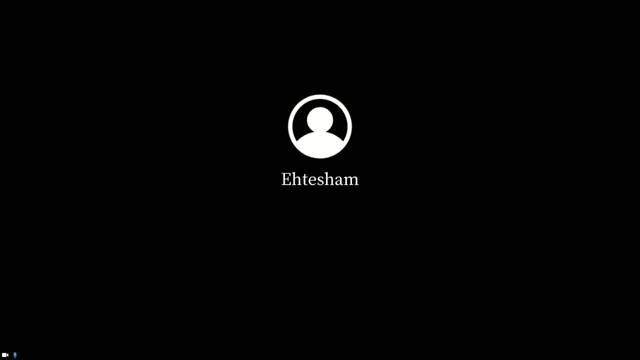 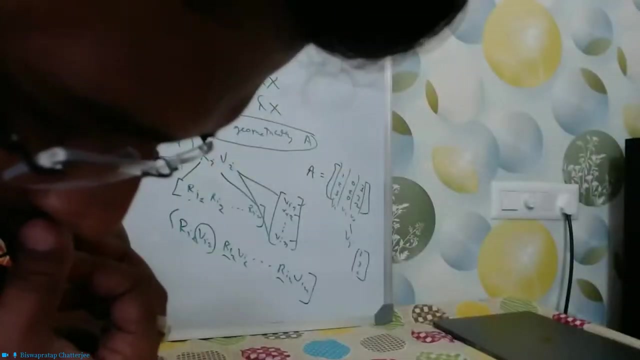 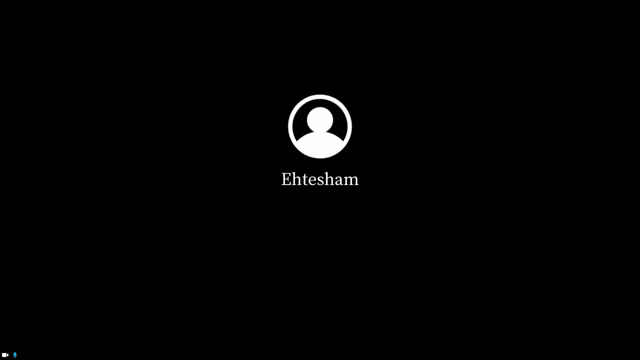 A minus I lambda is dependent on A minus i delta don't have inverse, so in that case we can't have elimination matrix. there is no guarantee that if you multiply an elimination matrix it still won't have an inverse. it may or may not have an inverse, but if you can prove it algebraically or geometrically, then great. 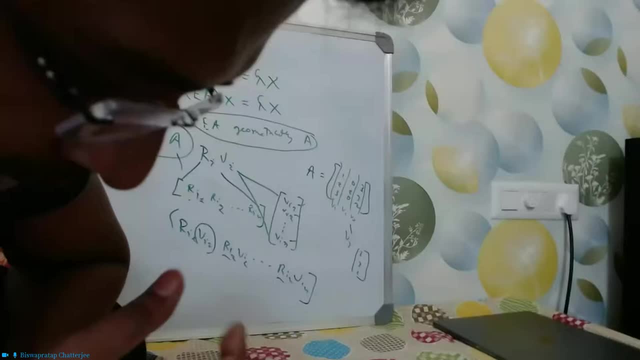 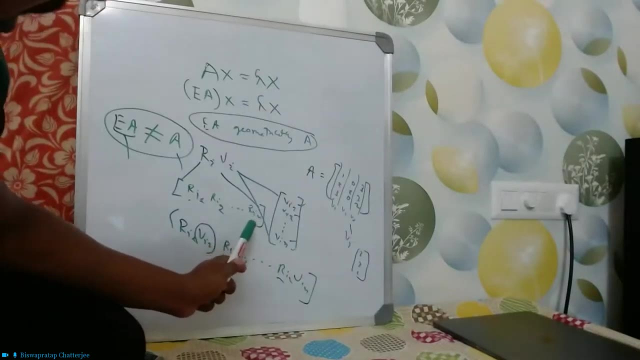 that approach is also fine but you have to prove it algebraically, like here. i proved algebraically that the v vector and multiplied by one of the rows of the ri vector, the elimination matrix, it changes because each of its components are scaled differently. so it kind of proves. 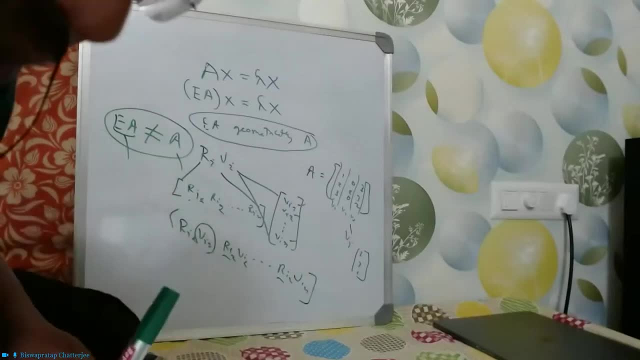 geometrically that my a is not geometrically equal to ea. so if you can prove that one in our inverse approach also, then also it is fine. but you have to prove it with a generic case. see here i used everything generic. i took n, i took any one. 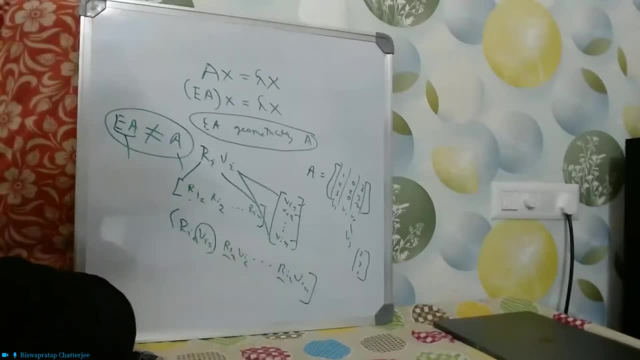 in between k and i use it. so this is the way to prove something without examples. so suppose you are doing a data science problem and there you found that a matrix is getting multiplied with your coefficient matrix, which you formed by the linearity matrix. so you can prove it. 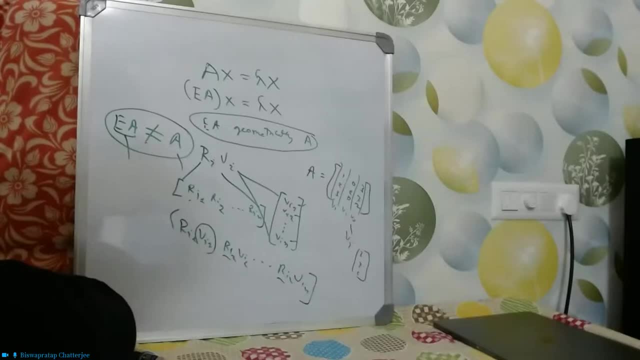 with a generic case. see here, i used everything generic. i took n, i took any one in between k and i used it. so see here, i used everything instantaneously. already doubtless you know. but and all of the data which isá glowing at the moment when you take a acids are not changingá. you can find many決. 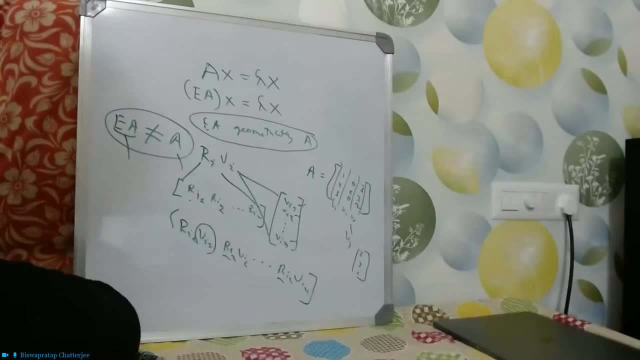 ignition of your problem now. you are not sureáthatáyour eigenvectors are eigenuns are changing orábecause if they are not changingáaccordingá here, taxes are not changingáwellá. if they are not changing now, what you can say that even ifrendreachingá alot of you know there is no, there is not any anythingáwhere in the world yif effects of the ancient past when we first question about, against the larger expression弊, if there are not changing and of 벌 Gmailá predictedÊthere are notchäng ha. 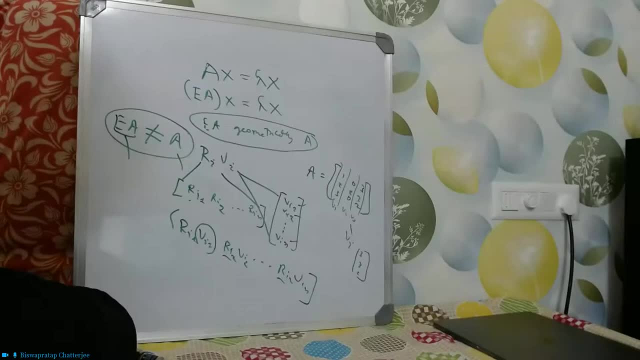 like yesterday, we did right a safety requirement of a car. okay, you generated the AX equal to B matrix. now that matrix, you found out that these are the eigen values, eigenvectors. according to that, you did your PCA and SVD decomposition and you proceeded with the solution. now somebody says that that I have. I have an. 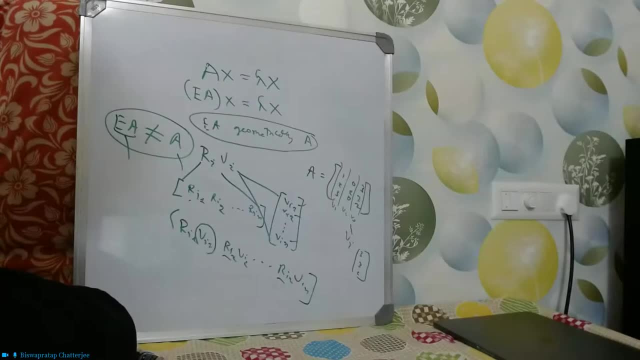 upgrade for this machine. okay, I have an upgrade for this car and the upgrade is represented by this matrix. so when you multiply this upgrade with this matrix, then your coefficients or airbag coefficients for breaking, coefficients for speed control options for auto steering, all these things values will 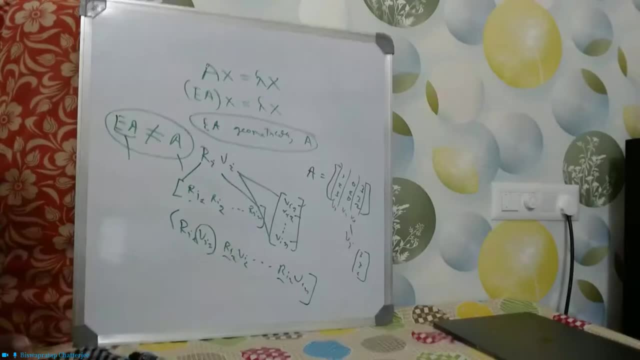 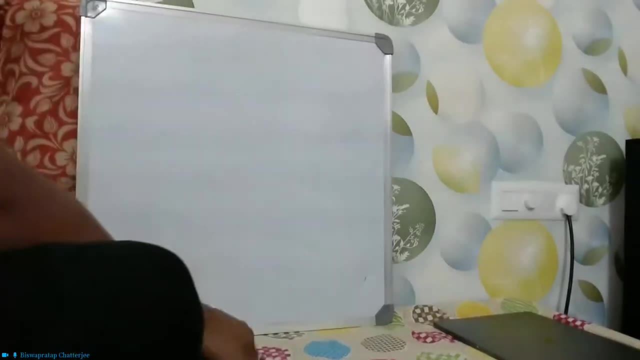 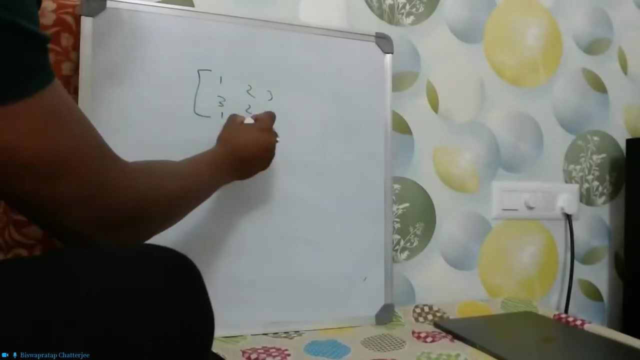 change right. so if I can show you it in a question form. so yesterday you guys did it right, so like you use this one, it was like one, two, three, three, two, one, one, two, one. so this was your say coefficient matrix of your car's safety system. now, 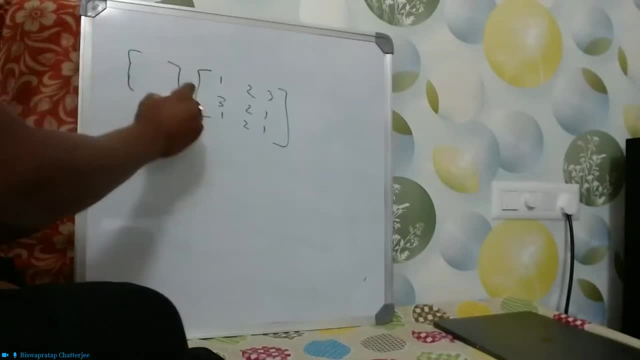 there is an upgrade and that upgrade is like a another matrix. okay, one zero one. one zero one, zero zero. say 0, 1 0, 0, 1, 0 and 1 0 0, 1. so what? what does it mean that this is? this is 0 and this 0. so the second row does not change the third row. 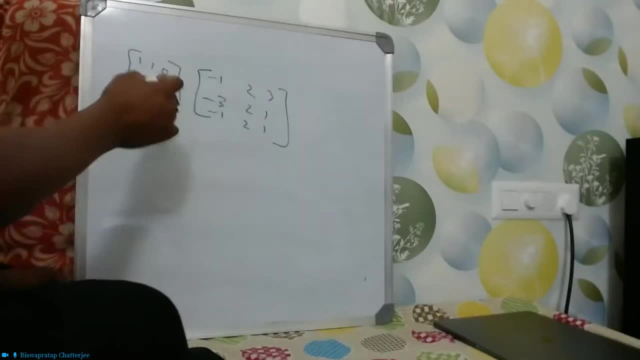 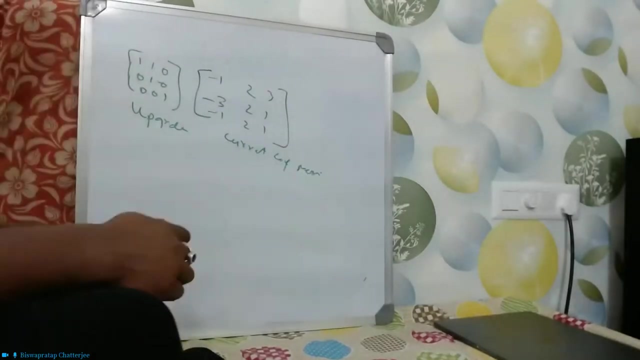 does not change, but the first row is an addition of the first row and second row: okay. so this is suppose an upgrade upgrade matrix. okay, and this is your current coefficient matrix. okay, so you say that if you upgrade by this engine, then your- and this one represents is, say, a: 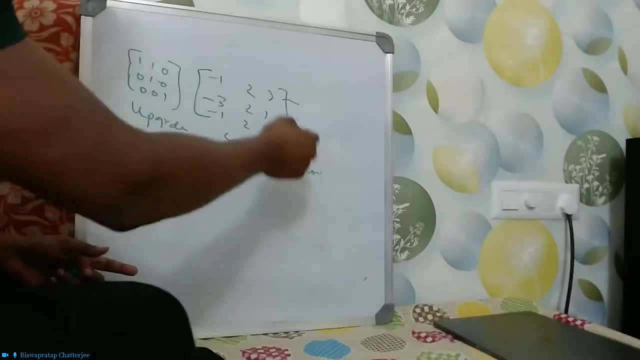 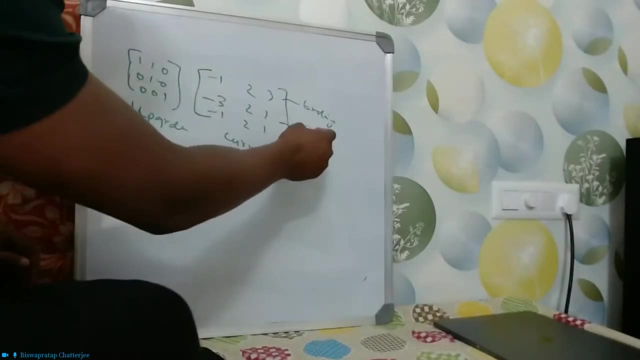 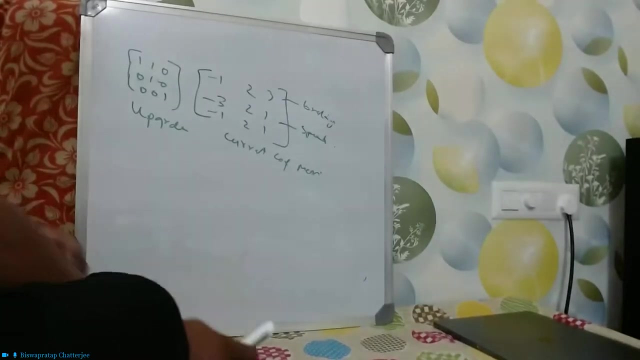 change in is represented or not, the change in the difference in your impact difference. in yourelsius, which is usually 7 Mantra, it will be same as in cathode force of the car. so right, so inunsure, take at 0.5 you 0 goes out, it means 0. you put about 8 sekarang. 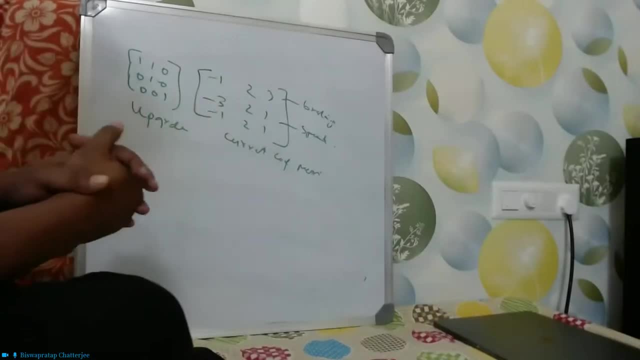 exactly okay, because now it is the third row here. 5 is its fault. very often this one get maybe 1.1 is the. they found out technical relationship between speed and brake and they said that when i upgrade, when you upgrade it, these two gets added and the new uh and the new matrix, coefficient matrix of. 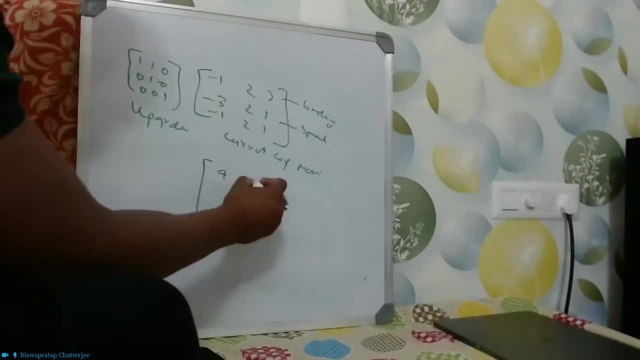 your car safety coefficient matrix is four, uh, two to four, three and four and three, two, one and one, one, one, two, one, okay, so what is this? one r1 plus r2, because r1 plus r2 is there, okay, and the other things remain same. so you say that this is upgraded. upgraded, uh, like safety features. 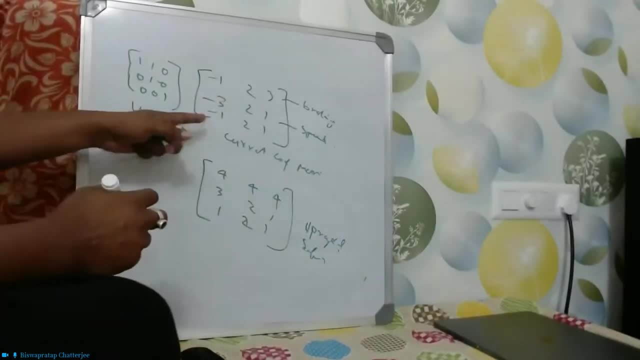 now you had solved everything using this one. okay, you had done the hbd decomposition, pc decomposition, everything. you had your eigenvalues, eigenvectors. depending on that, you did so many calculations. now, when you multiply this upgrade, so whether you can be sure that you need to recalculate all those things, and not because if 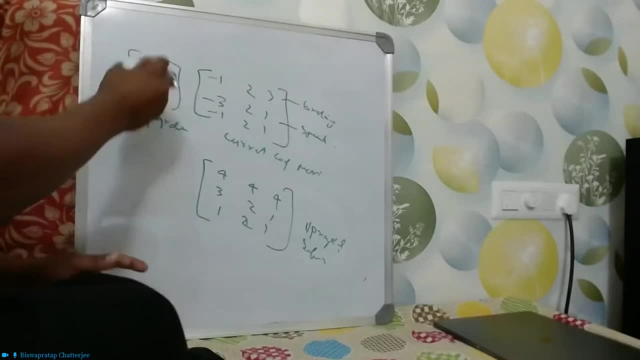 am multiplying a, just a unit matrix here. okay, i tell the upgrade. if you multiply, nothing changes. it remains the same. then you don't need to change anything because your machine has not changed. or you multiply a scaling matrix, all are same. two, two, two. then also your eigenvalues and eigenvectors. 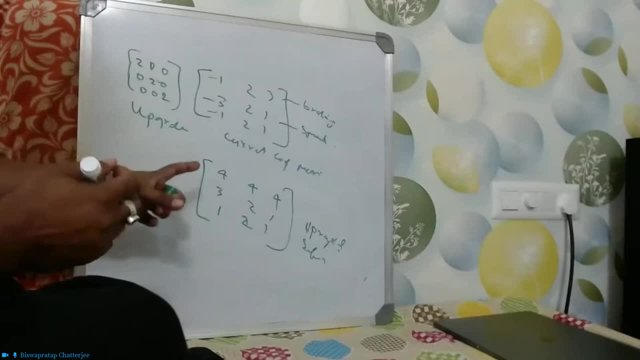 don't change right, because you scaled everything two times, speed breaking, uh, comfort. everything you improved two times. so your eigenvectors and eigenvalues don't change right, so your all other decompositions, everything don't change. so you don't have to do an upgrade on the entire model. 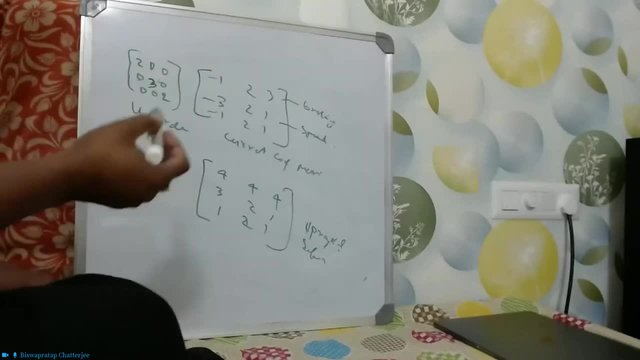 but if it is different, it's like two, three, two. then what happens? you, you, you tell if you know that if i multiply a elimination matrix with this one, or a matrix product of this format with this one, then my eigenvalues will change. um, then, in that case, what? 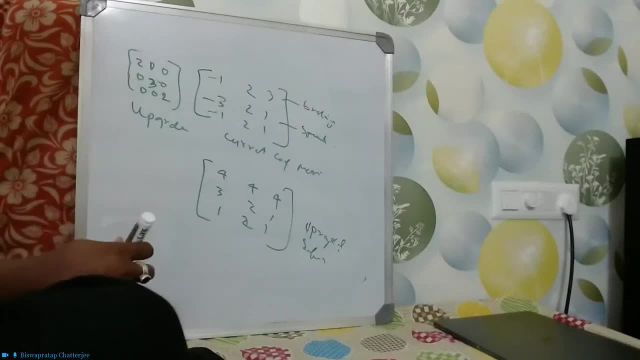 you will see is that if i multiply a matrix with this one, or a matrix product of this format with this one, then my eigenvalues will change. then, in that case, what you do? you need to recalculate and reevaluate your model. okay, this is a use case i am giving of the 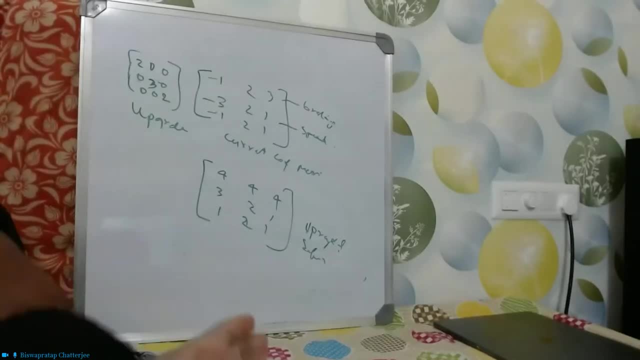 question i gave you. okay, so, so there are some special matrices which may occur very, very frequently in the nature of your solutions. so one is identity matrix, one is elimination matrix, one is a permutation matrix, one is a rotation matrix, one is a projection matrix. okay, projection matrix. 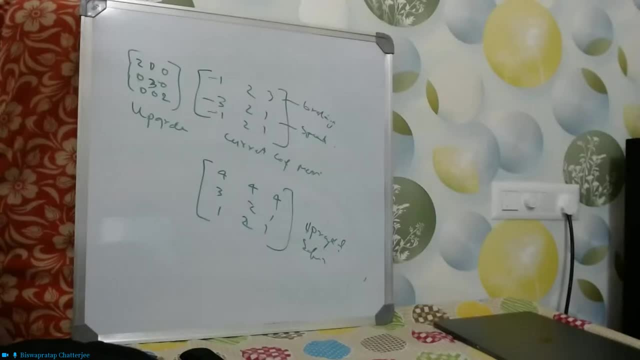 is not read until now. but rotation, elimination, permutation, uh, and identity, all these metrics and scaling matrix, all these metrics you have already read right. so now these matrices very often come in your path while solving the data sense problem and they get multiplied with your original coefficient matrix and change it. so you, if you by hand, know that, oh, this is. 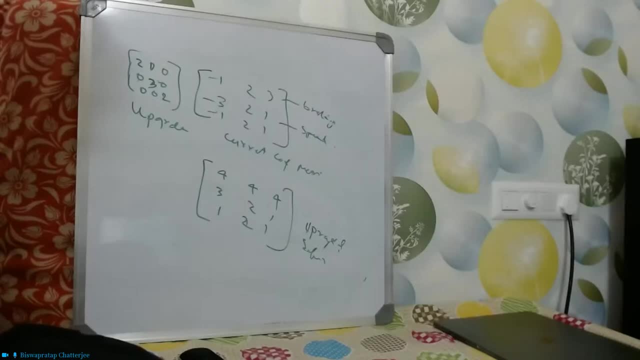 kelly matrix. okay, though, okay, the eigenvectors and eigenvalues don't change, so i don't have to to change anything. so mathematically you know that it's not affecting your solution, your model is still holds good. but if you don't know, then you will be always in doubt. what happened i need? 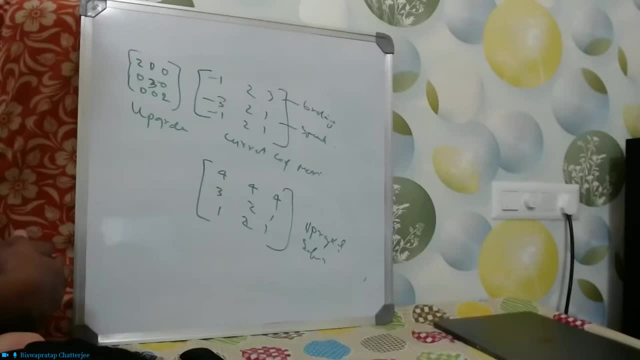 to recalculate, so you will recalculate when ultimately, you will see that, okay, no change was there. okay, so these are the use cases of that's why i gave you these multiplications. if you know new projection, i would have also given projection matrix multiplication. but so these are the three. 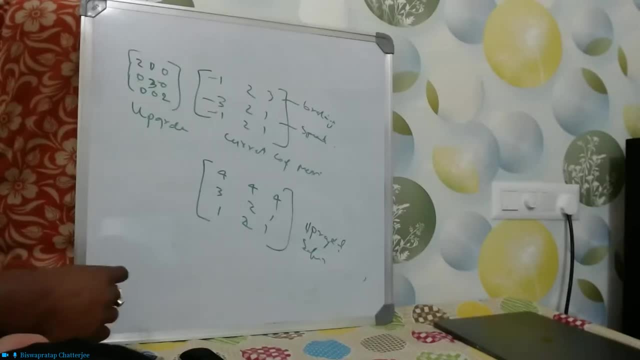 and one more thing to learn from here is- this is the conceptual part- that why i am doing this, okay, why i am testing that multiplying these matrices with my coefficient matrix has any effect on the eigenvalues or eigenvectors. this is the conceptual explanation that i gave you. 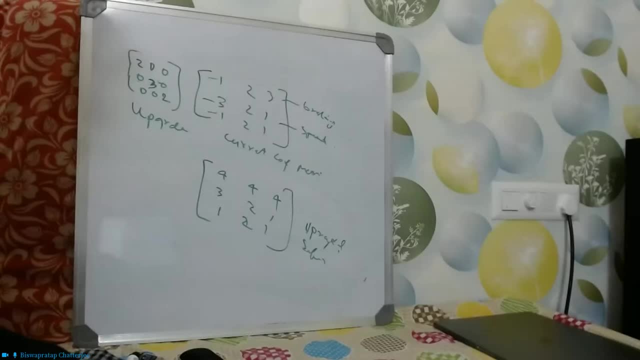 why it is a mathematical way or approach, how to do it, how to confirm yourself is done. by the way, i showed you how to generically prove that or disprove a particular assumption. So you cannot tell that I have this matrix and then I multiply. So there can be a situation where that elimination matrix is such a design. 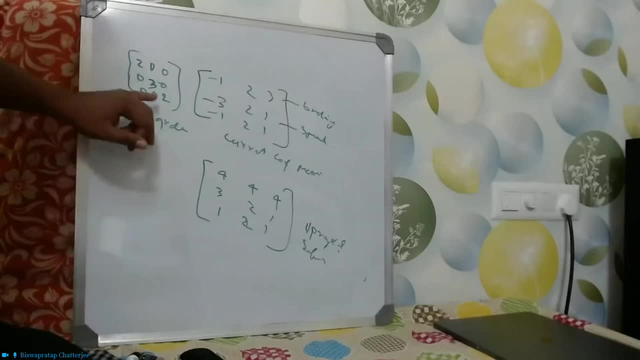 that everything scales up equally. So if this is the elimination matrix, in case of 3, I write 2.. If this is the elimination matrix, then obviously your eigenvalues do not change. ok, Vectors also do not change. But if my elimination matrix is like this, ok, then 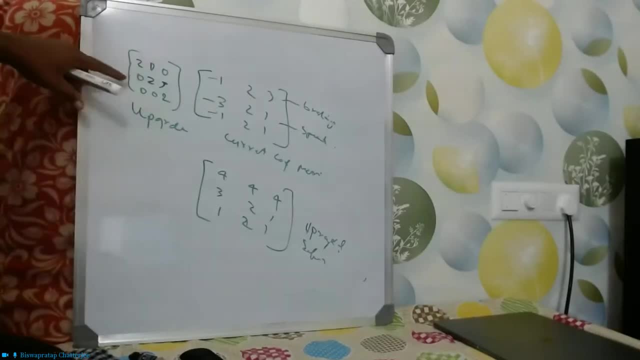 it definitely changes. ok, I am. so this will become Rk. This Rk will multiply with- sorry Ri. This Ri will multiply with Vi And in Vi, each component. the first component will be zeroed out, The second component will be increased 2 times and the third component. 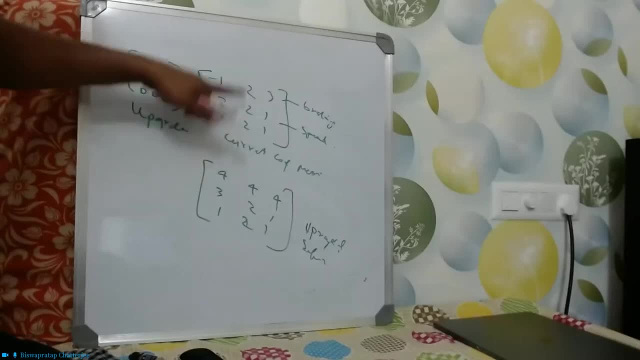 will be increased 3 times. In that case, my this Vk Vi completely changes. Since Vi completely changes, the eigenvalues and eigenvectors of this also changes. So I can no more rely on this new coefficient matrix. I have to recalculate. 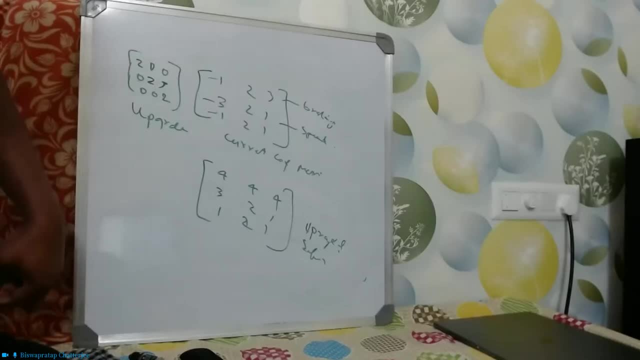 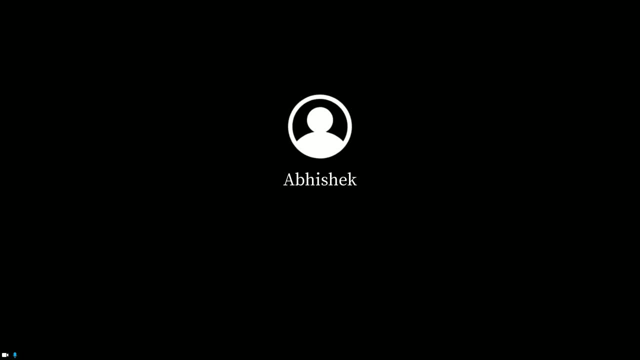 Are you alive? Yeah, yeah, yeah, yeah. Ok, And Ayyappa-shaam, are you here? I am going out to the doctor. Huh, Abhishek, I am going to meet the doctor at Vishwavata. 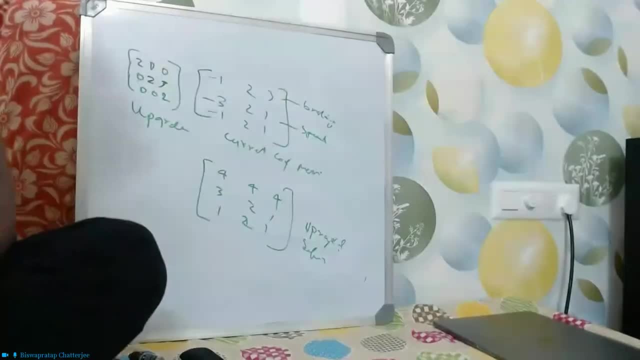 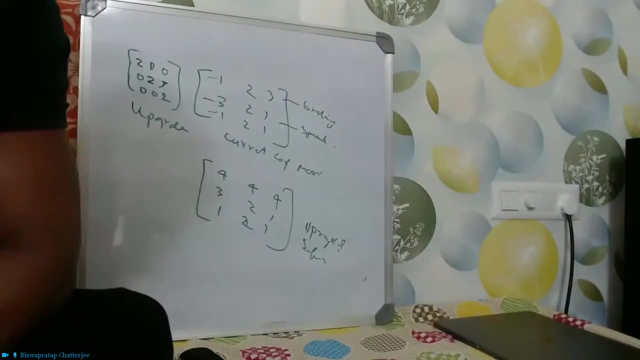 Oh, ok, ok, You can leave, No problem, Go go, This is anyway recorded, You can see it again. Yeah, I will check it. Yeah, Ayyappa-shaam, Yeah, Biswa, I am here, I will try to solve it. 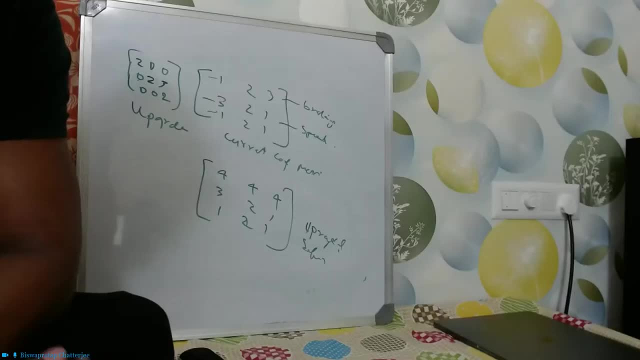 You are clear on what I did here, how I proved it. Yeah, this I got. yeah, Ok, So same same way. try to prove or disprove that, whether, when a permutation matrix is multiplied with a coefficient matrix A, whether